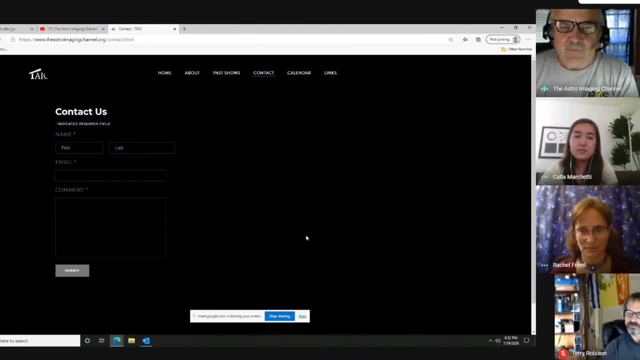 but we just figured we'll make a little PowerPoint of all the comet pictures. This is also, incidentally, the place where you can send us stuff about if you want to present something, if you've got something that you have been working on that you would like to. 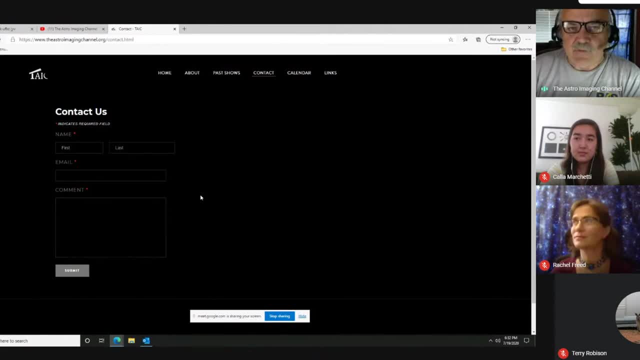 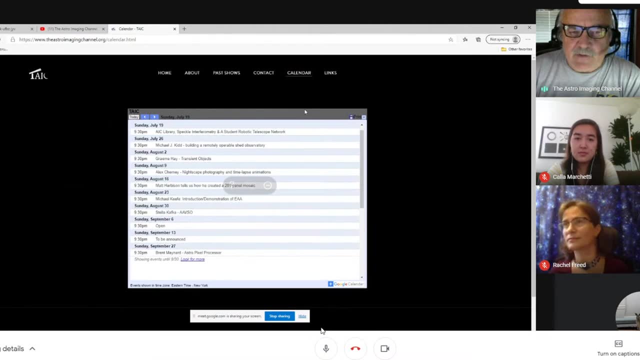 share with the Astro Imaging world. Well, this is the place where you would put your name in. to do that, I always take a moment or two here to tell us about. you know what's going on in the Astro Imaging world. I like to talk about what's coming up. Obviously, today we've got Rachel and Carla. 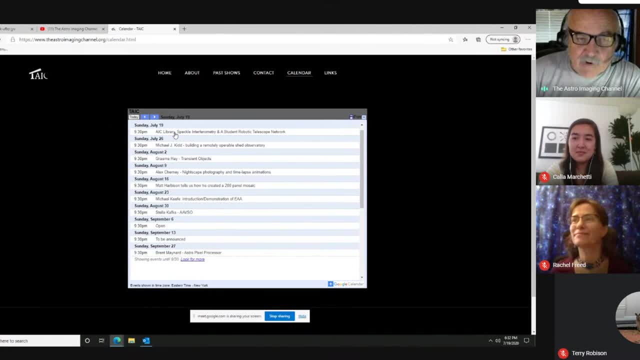 and Ryan and they're going to be telling us about the AIC library. Remember, AIC really stands for the Advanced Imaging Conference. TAIC came along later and they are not AIC. different operation, All right, But they've opened up their video library of all the presentations through the. 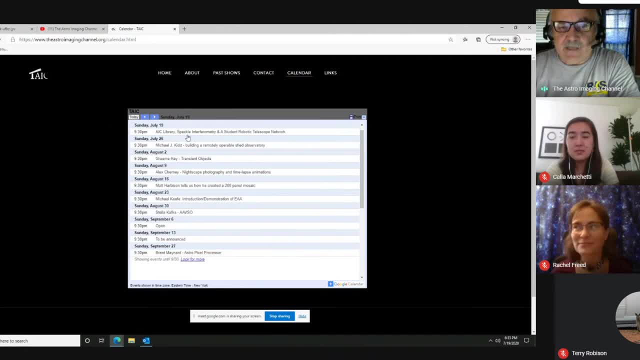 years And Rachel's going to tell us about that. And then Carla and Ryan are going to get together and they're going to tell us about some of the projects that they've got going in Astro Imaging. My kid's going to be here to tell us about building a remote operating shed observatory. 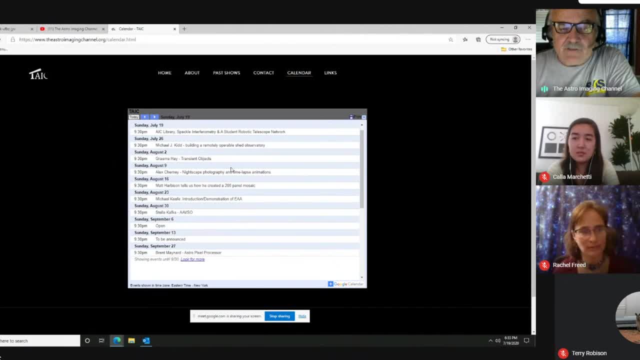 Graham Hay is going to be doing transient objects a week after that And Alex Cherney is going to come along and tell us about nightscape photography and time-lapse animations, And we're pretty much scheduled for a while. here We've got some opens and to be announced. 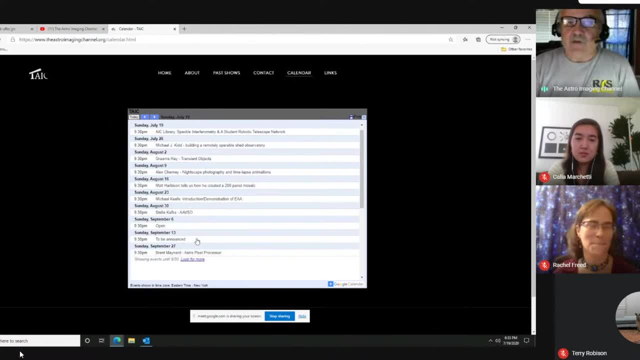 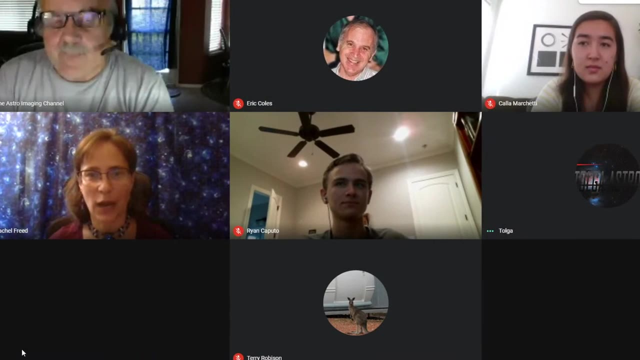 coming up in September. We would like you to help fill them. if you can do something to spread your Astro Imaging knowledge, It would be of great value to us. Okay, With all that in mind, I'm going to stop sharing my screen and get back to you. Rachel is here. Rachel comes to us from 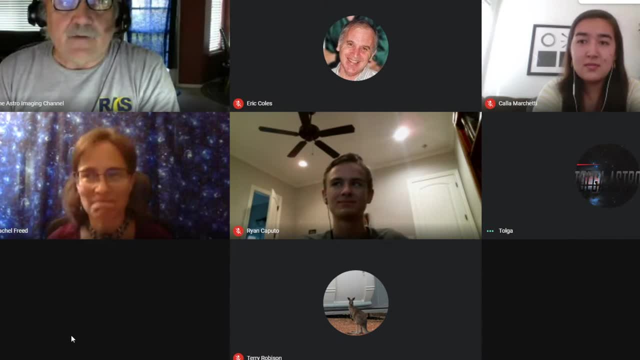 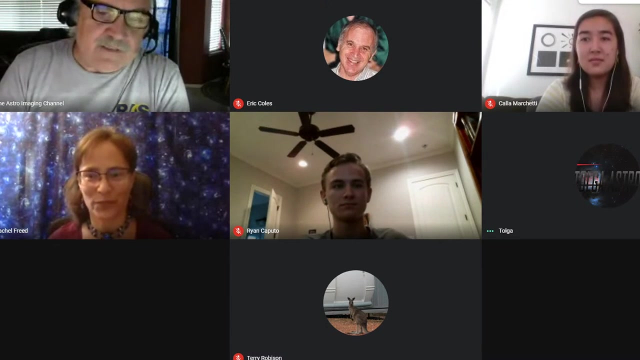 she's the newly elected member of the Board of Trustees of the Advanced Imaging Conference And she stepped in at the last minute. You probably heard me say last week that our presenter- scheduled presenter for this week- couldn't be here, But Rachel stepped in, volunteered and brought 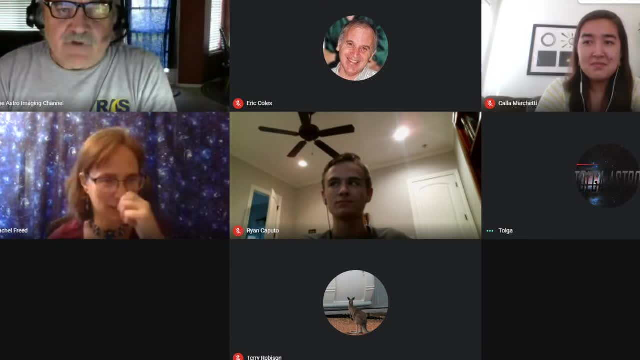 along a couple of people that have been working on some projects, So I'm going to let you take it, Rachel. if you can take it from here, Go ahead All right. Thank you so much. I'm excited to be here again. I was here in September. 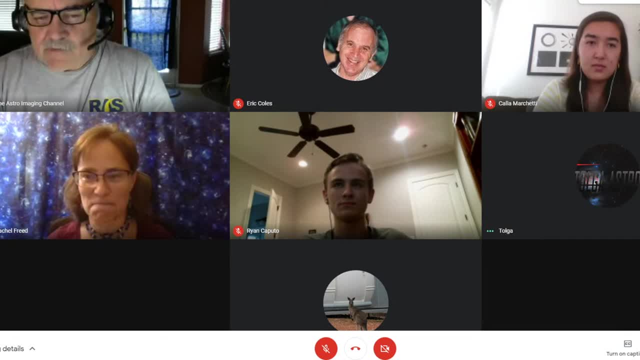 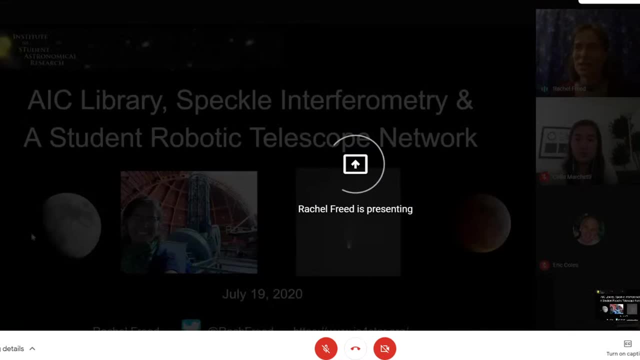 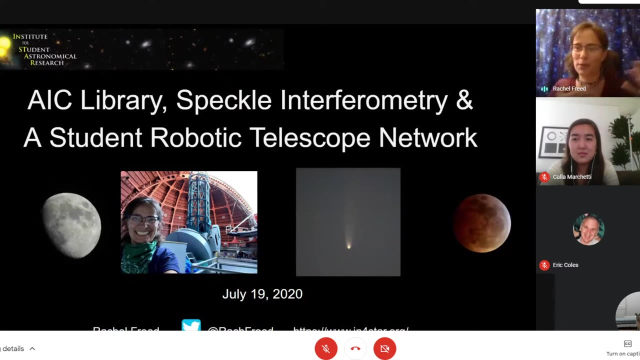 And let me share my screen. So we're going to be talking to you about a couple different things. today. We're going to be talking about the AIC library, and I'm very excited to be on the board of the Advanced Imaging Conference, And then we're going to talk to you about projects that Ryan and Kelly are working on. 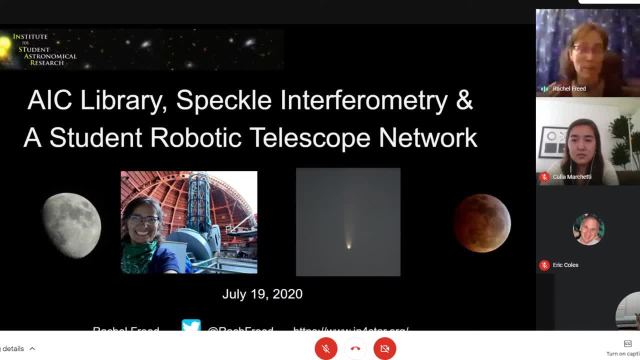 And I want to just put this in a little bit of context. So about me: I work with students around the country and educators- college instructors, high school teachers- to help students and teachers get involved in astronomy research. And there is, of course, a lot of tie over between research and imaging. There are people who start out. 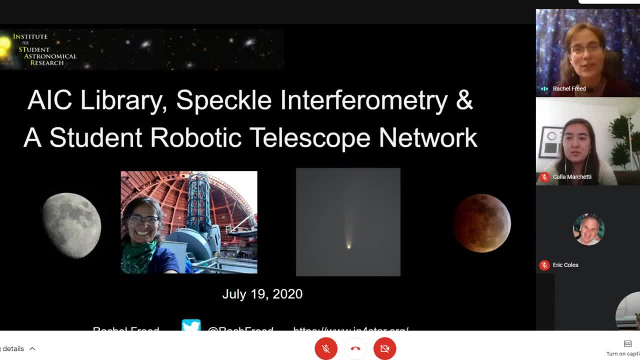 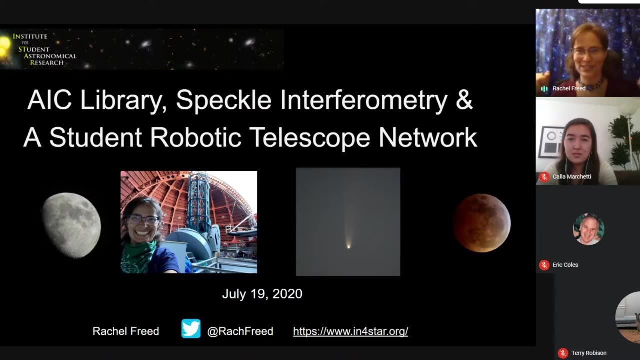 in imaging and go into research. There are people who are going to start out in research and go into imaging astroimaging, So these are, of course, very related, And a lot of the work I do is bringing together these different communities, these research and education community with astroimagers, so that we can all just do more cooler things. 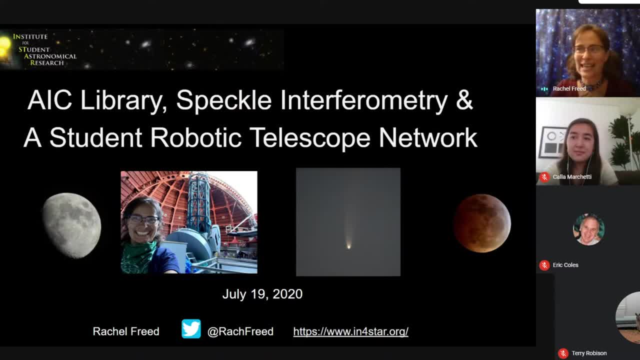 together. So I'm going to talk about the AIC library and then they're going to talk, they're going to take over. But I just want to mention I'm the president of the Institute for Student Astronomical Research. There's a picture up here showing me at Mount Wilson. that ties into the research. 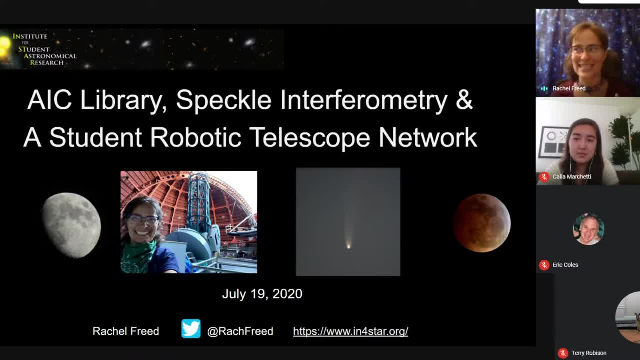 program or the research that Calla and Ryan have been doing. I'll get into that later- And of course, I had to put up my comic picture. It's not the greatest, but it's what I can do with what I have. So one of the things that I always keep in mind. 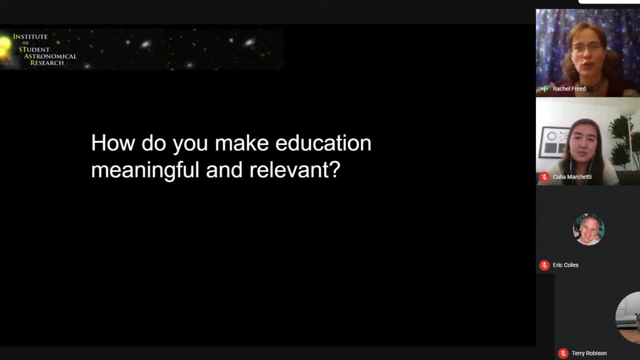 in. everything I do is how to make education meaningful and relevant, relevant to students, meaningful, interesting, And actually I work with not just students, not just teachers, but I also work with people who are interested in the research, not just researchers, but people, anyone that's interested in using telescopes for research or imaging. So, always in the back of my 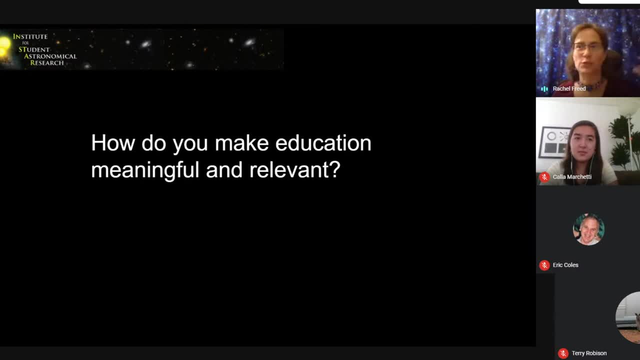 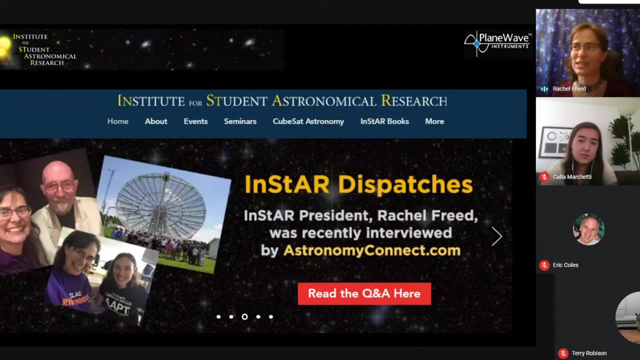 mind, And so I want to have that be sort of the lens with which we think about all this today. How do we make education meaningful and relevant? And so I co-founded, and I'm the president of, the Institute for Student Astronomical Research, And under that umbrella I teach a lot of. 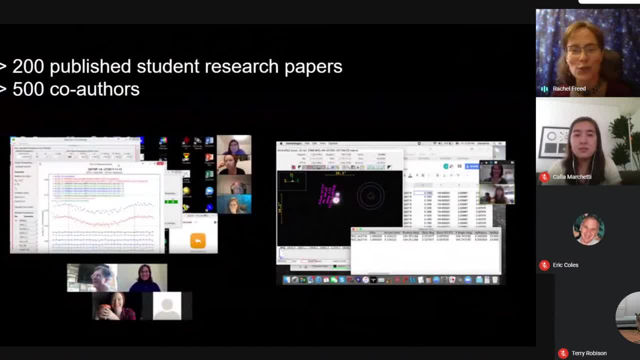 astronomy research seminars And I just we've been using Zoom. I know it's really fashionable now, even though I guess we're on Google, but we've been using Zoom for years for our program. But over the past 10 years we've had over 200 published research papers with 500 co-authors of you know. 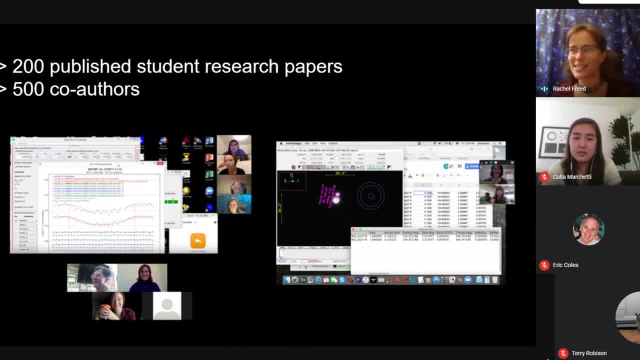 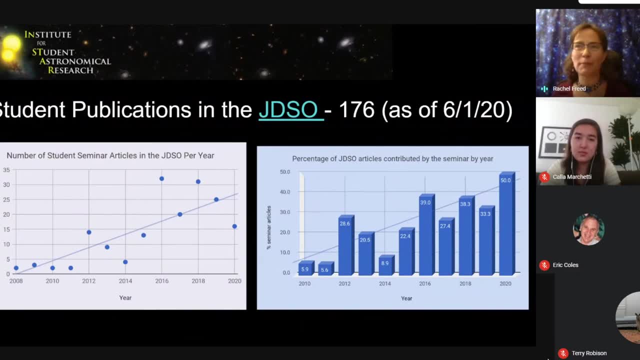 students, ranging from eighth grade up through graduate students, And that's that's sort of my, my focus in life. We publish a lot of our work in the Journal of Double Star Observations And, as of this year, 50% of the articles that are now published in the Journal of Double Star Observations come from. 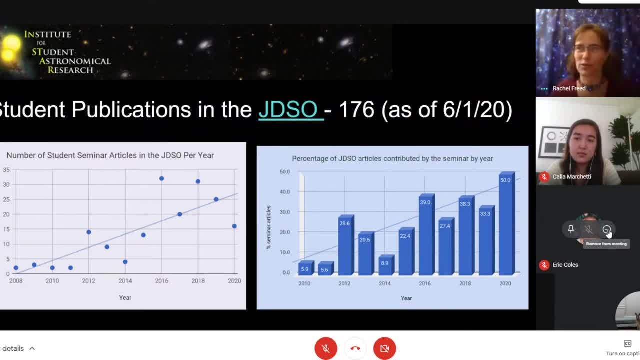 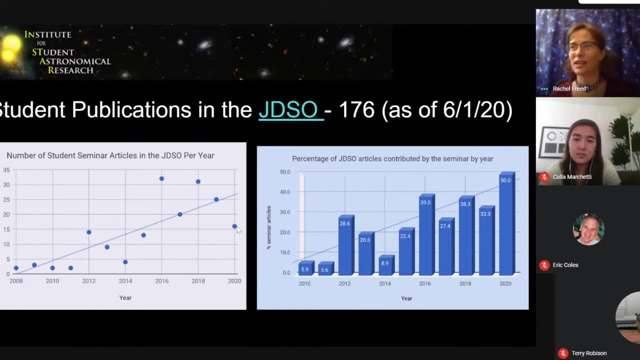 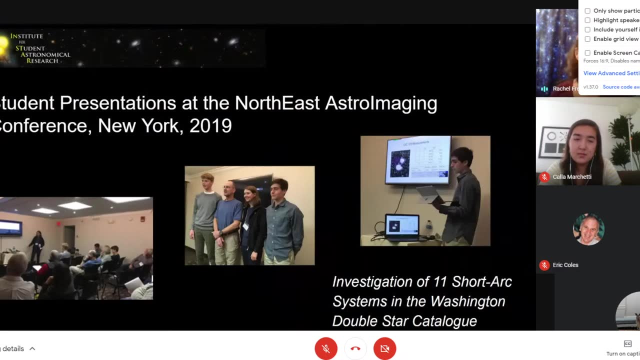 students doing astrophysical research Within the sort of structure of the astronomy research seminars that I run. So that's really exciting. So we're up to halfway through the year, you know more than 15 published papers and I think we're on track to at least have 35 this year. That's exciting And I have students I try to provide. 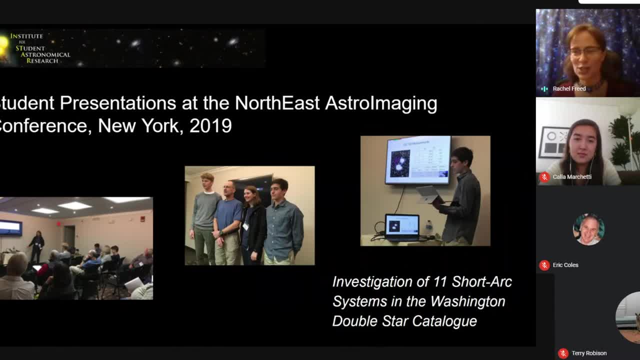 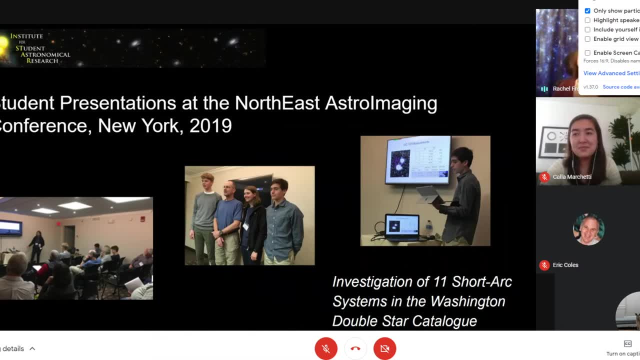 opportunities for students to present at all the conferences I go to. It just occurred to me. I made this an opportunity for students to present research. That's exciting. So we had. we had students that presented at NEAC last year. we would have done it this year. but 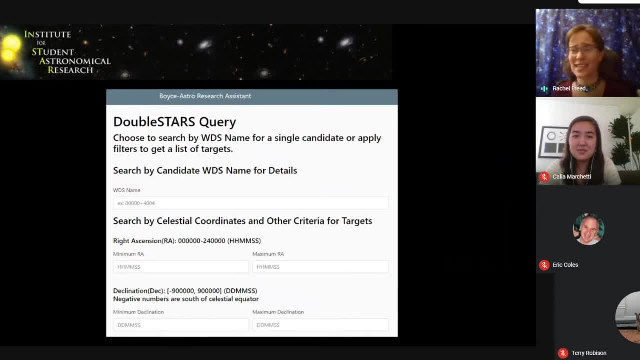 well pandemic And we have students that take it further. they do research and then they say: you know what we need? a better online browser based search for double stars to research. and they build it And you're going to see what Calla and Ryan have sort of taken on in this, starting out with research and then just doing more, and 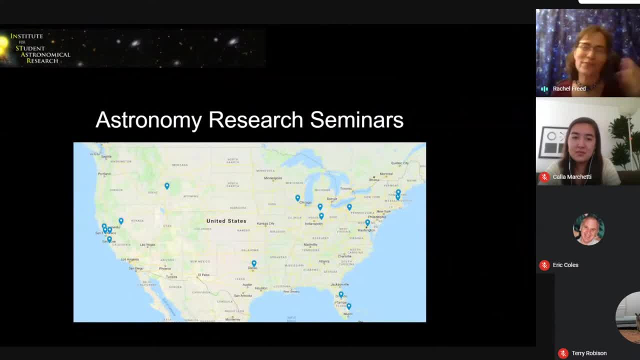 more And it's really amazing And our programs are all over the country And that's really exciting. And actually I'd say this map is now six months old and there should be lots more dots on it. I'll have to update it. 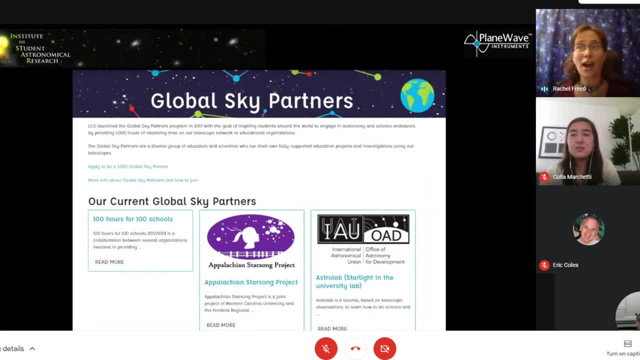 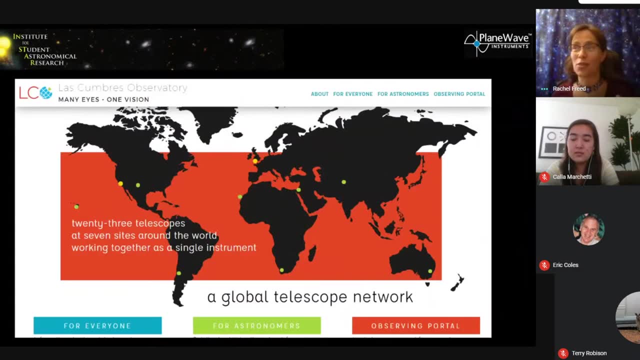 I'll have to update that map, But it's really exciting work And we are one of the global sky partners with the Alaska Race Observatory Telescope Network, So we actually get to use telescopes around the world, northern and southern hemisphere, And that's really exciting. 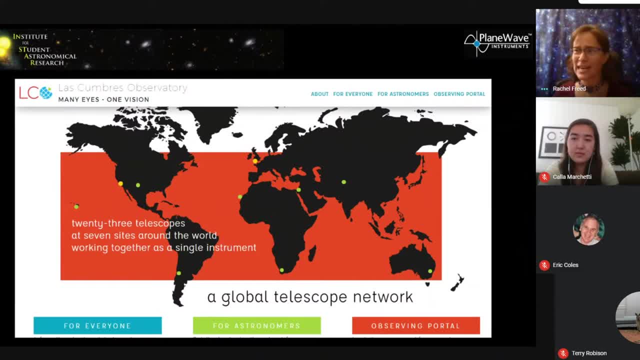 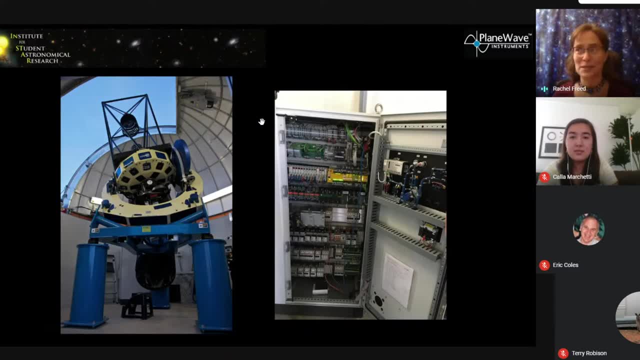 Yeah, the imaging opportunities are pretty amazing, And there's an example. that's one of the one meter telescopes that we occasionally get to use. Normally we're we're limited to the point four meter telescopes, but it's fun stuff. 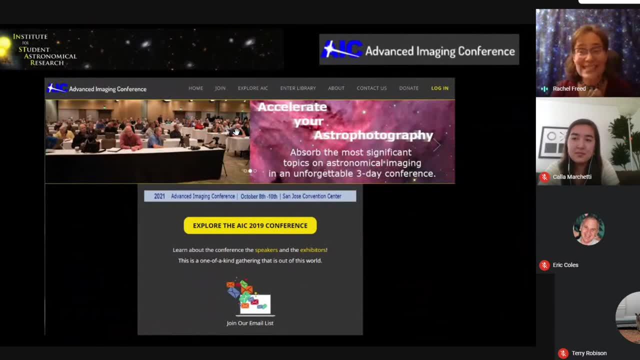 So what I want to talk to you about right now is the Advanced Imaging Conference, And if you have not been to the Advanced Imaging Conference, I am going to encourage you to come out. It's it's we have over a year from now, So hopefully by then we can all get together in person and things will be safe and open again. But October 8th to the 10th 2021 at the San Jose Convention Center in California. 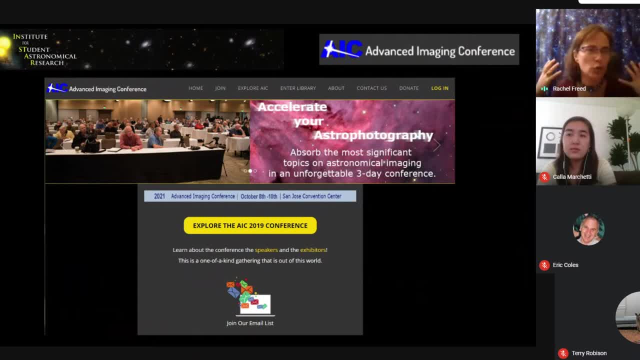 So here the Advanced Imaging Conference really started out as a group of people that were interested in imaging and wanted to get together. So here the Advanced Imaging Conference really started out as a group of people that were interested in imaging and wanted to get together and share their knowledge with each other. and it's grown over the years, over 15 plus years. 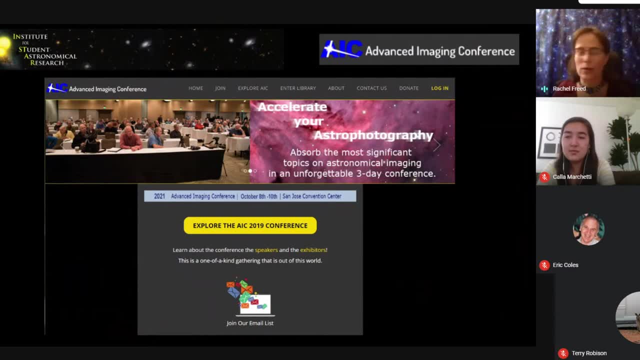 And there are talks, there are workshops where you can get into great detail about how to use PixInsight and all the other things, And I'm going to show you some of the past workshops that have taken place. But what I really want to mention is they decided to make their library of recorded past workshops and talks freely accessible to the public. That's all of us. 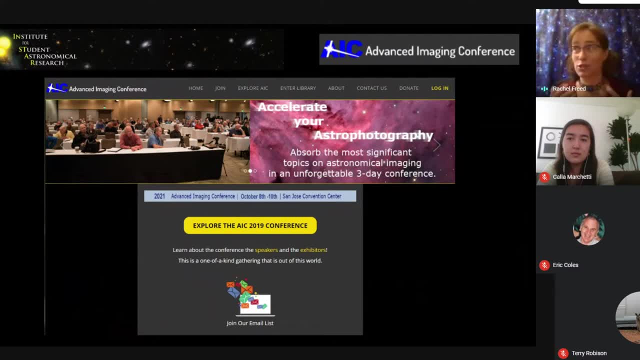 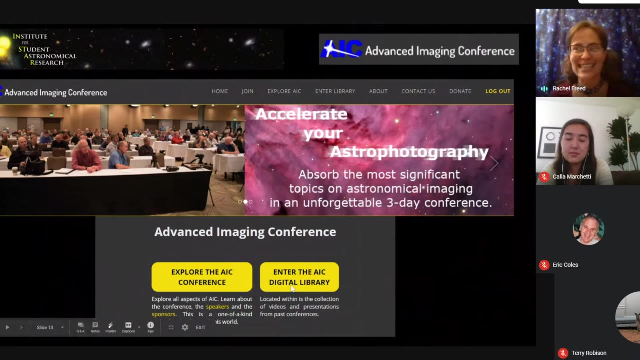 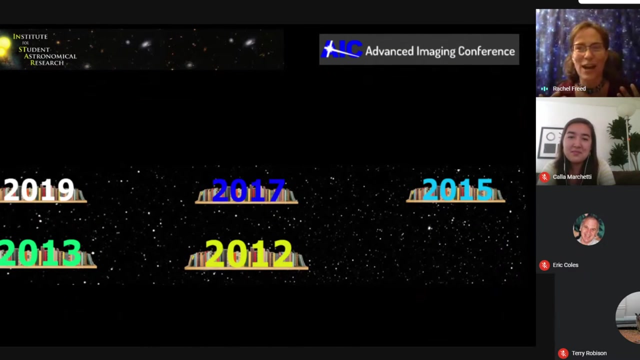 You do need to become a member, but membership is free. Just go on their website and click the login button. make yourself a member for $0.. That's a great price to have access to all this stuff And once you are logged in, you can. you'll see the enter the AIC digital library. Okay, this is where it gets exciting, you guys. Okay, so they have their- all their recorded presentations from 2019, and the conference now happens every two years. 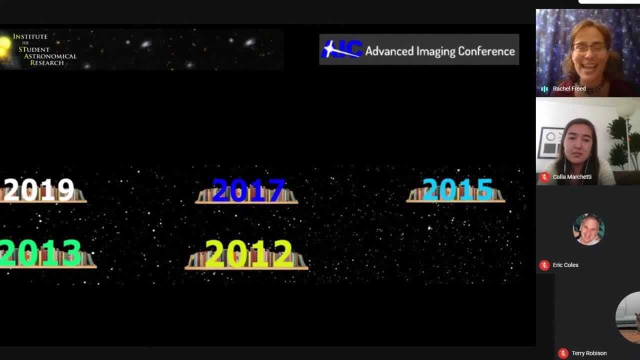 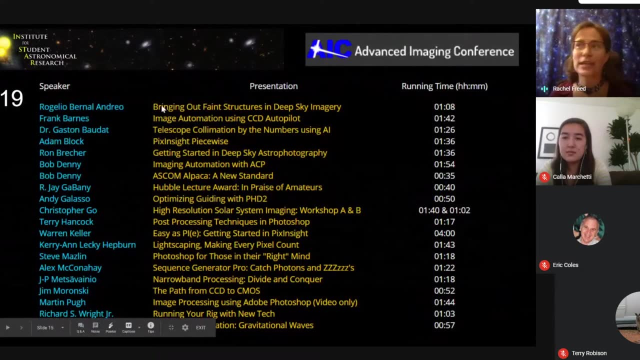 So 2017, 2018, et cetera. So let's take a look at what are some of the things that people talked about, that you can go and watch their videos- So bringing out faint structures in deep sky imagery- So cool. In fact, they often have award. they have actually every year award ceremonies at the conference and they bring in people that have done amazing things- And I got to see a talk. 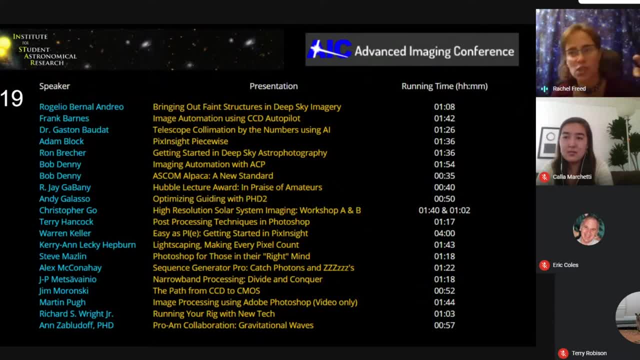 two years ago. I think that was just incredible about finding these star streams in galaxies from doing super deep imaging and it was really phenomenal. But telescope collimation, There's a lot about PixInsight, So I know I'm speaking to a bunch of astrophotographers and if you're really interested in getting a little more information here, you know digging deeper with Sequence Generator Pro or 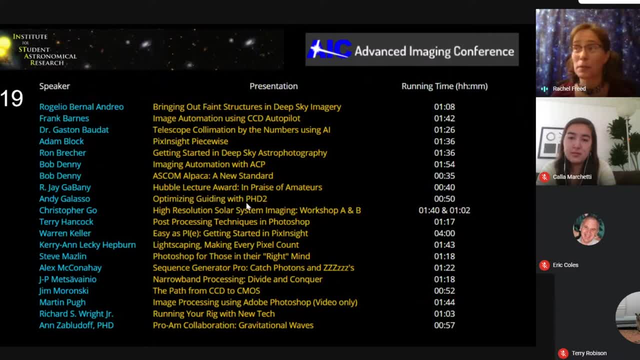 there's a lot of PixInsight here or guiding with PhD2 or Photoshop. So these it tells you how long the videos are. What's also great is if you click, you can watch them. So if you click on the top of the video, you can learn about who all of these. if you don't already know who the speakers are for each of these, you can just click on their. 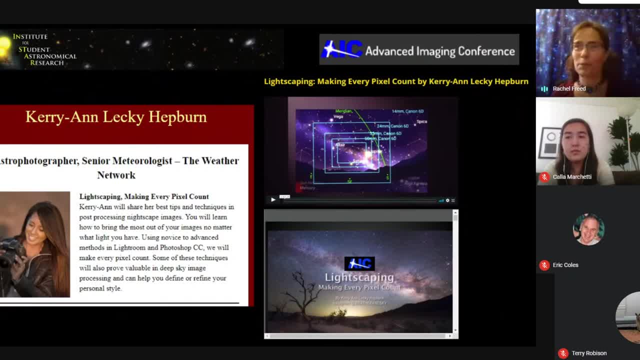 names and see what what they're about. For example, Carrie Anne. she was one of the speakers the last few years And on the website, not only do they have the- in this case, an hour and 43 minute long workshop that Carrie Anne gave, but they also have for you to download her slides in a PDF format, So it tells about the speaker. 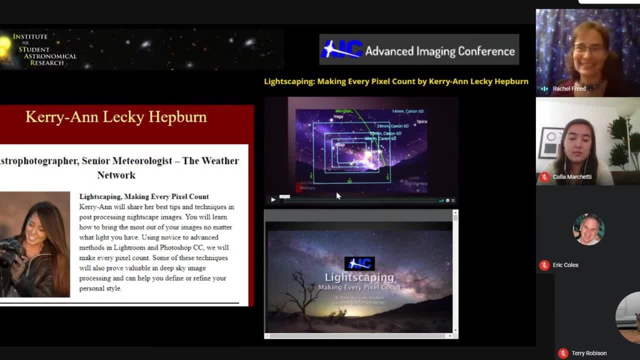 has their whole workshop right there for you to really learn from and you can download the contents. they don't have that for all of them- the the contents to download, but a lot of them they do, so that's really cool. um, so i want to go back to just look at a couple more of the topics. um. 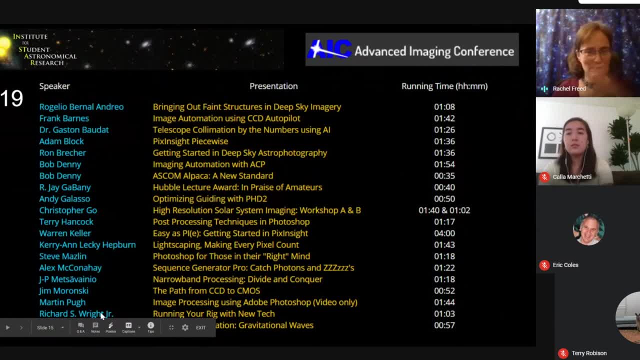 running your rig with new tech. richard wright- probably everyone who knows who richard wright is, um the path from ccd to cmos. that's actually an interesting one. that's applicable to what you'll hear ryan and akala talking about tonight. um, and let's see. so, carrie ann she's, she was there. 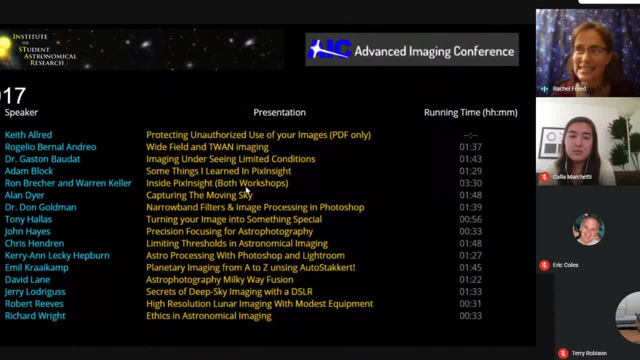 the, the conference. before that, of course, picks insight. um imaging under seeing limited conditions. that might be a big issue for many of us. um secrets of deep sky imaging with the dslr anyway. so you can see that there's quite a range of topics here and it's all freely accessible to. 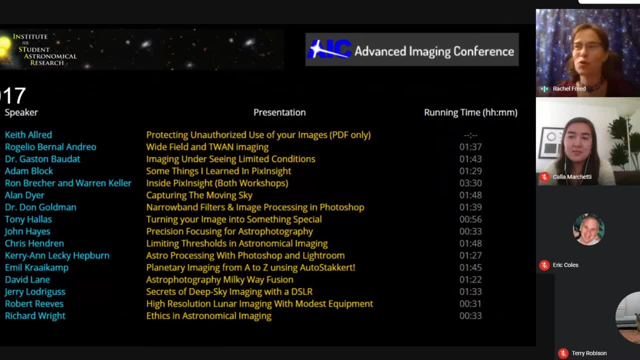 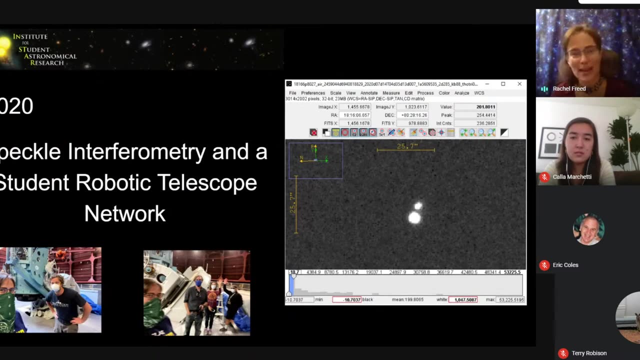 you and i would encourage you to go join the site, um, explore the library, learn more and come and meet us all in person at the conference next year in october, and um with that. so that's the advanced imaging conference digital library. please, you know, join that group and um join us. it's a lot of fun and um, there's so much to learn from each other. 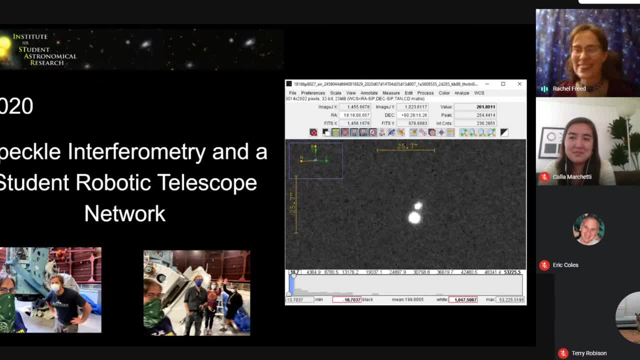 i love being part of this community, okay, so, um with that, i want to just briefly mention, um how what ryan and cal are going to be talking to you about how that sort of came about, i think. um, so they're going to be talking about speckle interferometry and a. 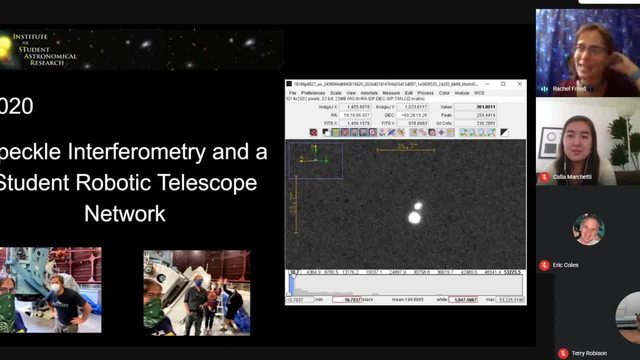 student robotic telescope network, so two sort of related things that they're working on together and um we, the institute for student astronomical research we usually hold, we've started holding seminars for students up at mount wilson, but this year and we get to use a hundred inch or 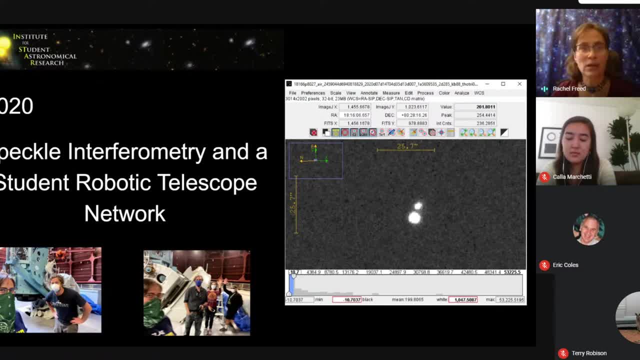 the 60 inch telescope. but this year, of course, with the pandemic, we had to change things up and we did it online. so we had these fake zoom meetings where we invited students and teachers, we invited adminisers to speak, um every spring they were able to open up their doors. they had 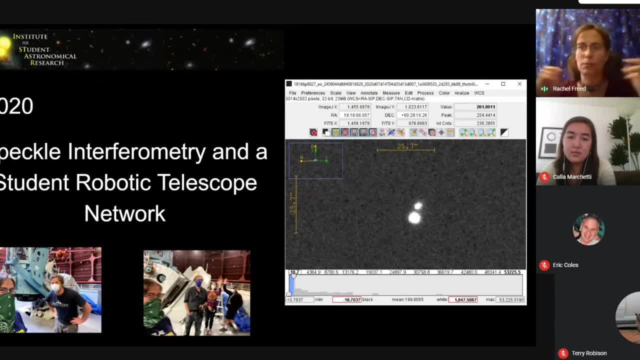 是不是 didn't have the need for augo? they didn't have to. is it open all the spots, all the collected speckle interferometry data which they're going to talk to you about, and they've now done a lot more speckle interferometry. This was just in May and now they'll tell you about. 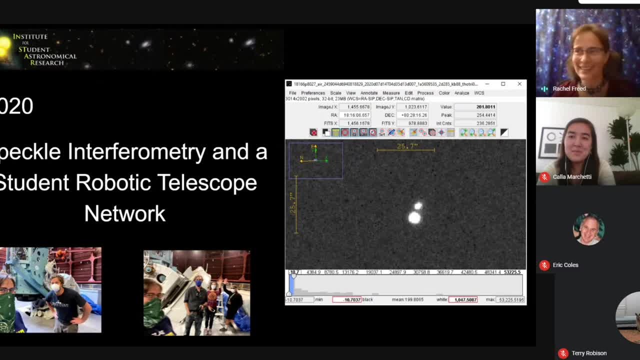 the papers they're writing where they've studied. I don't know more than 30 double stars, but what's so cool about speckle interferometry and you'll hear from them. the picture on the right shows a double star, and the reason we do double stars for research for students, is because it's a sort of 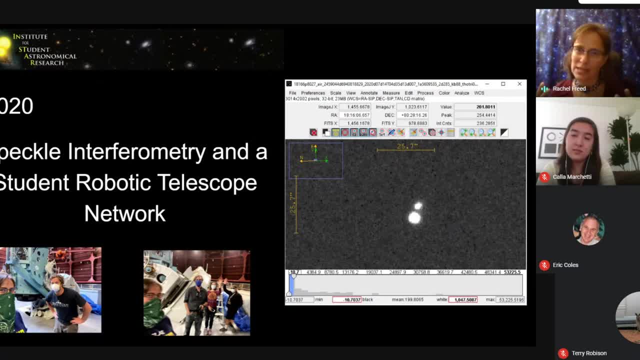 the simplest entry point into research into astronomy. It's something that's manageable in the small time frame that we have, and this picture is from one of the Las Cumbres Observatory 0.4 meter telescopes showing about as close a pair of double stars as we can actually resolve. 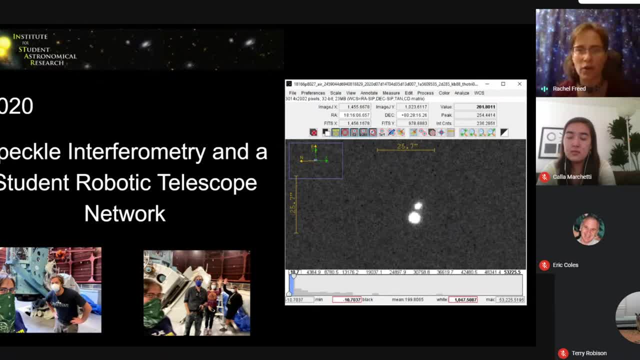 Those stars are about 5.7 arc seconds apart from each other, and that's about down to five arc seconds is the limit that we can sort of resolve with the 0.4 meter telescopes and the equipment from the Las Cumbres Observatory telescopes that our students have. 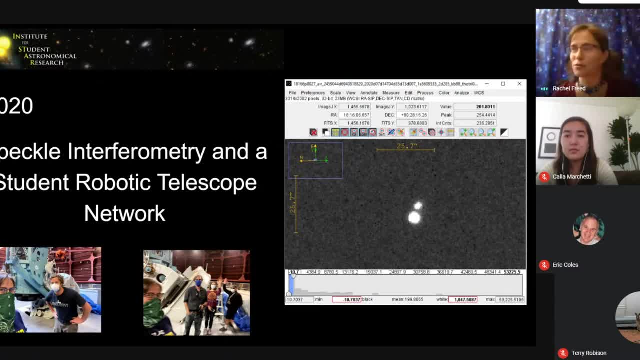 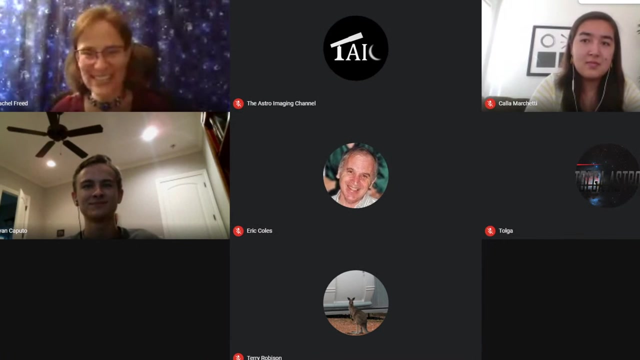 free access to, which is a whole other amazing program, but what Ryan and Calla are working on can get 10 times closer stars and it's awesome. so I think I'm gonna have Ryan and Calla take it away. I'm gonna stop sharing my screen and let you guys take over. so, Ryan, you can both turn on. 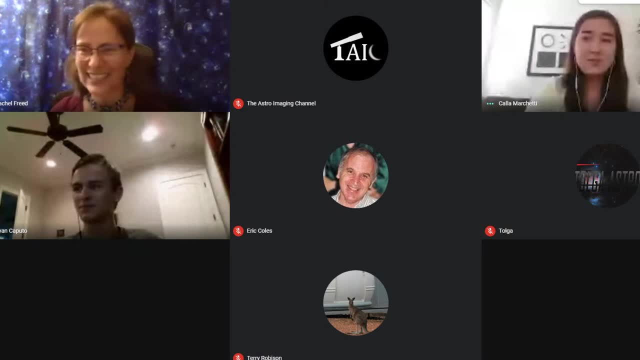 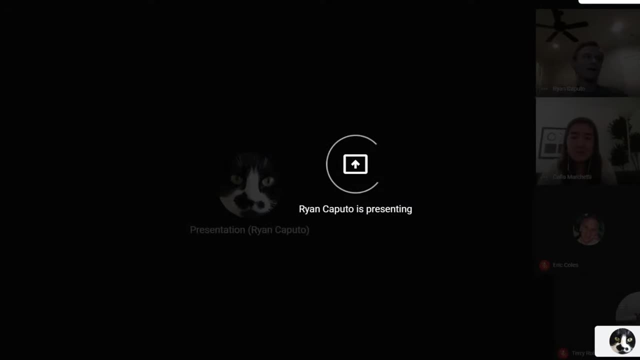 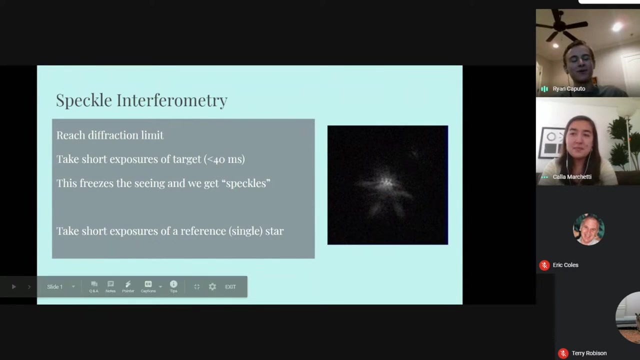 your mics. Okay, yeah, thank you so much, Rachel, for that wonderful introduction. We are doing double star and I first got into it a while ago because of Rachel and, well, specifically because of my astronomy teacher, Kalei Talk, and man, it's pretty addictive and the whole process. 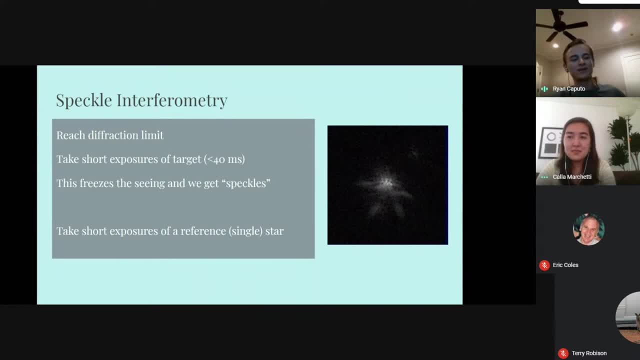 and I met Calla last year and she's been I kind of mentored her project and she's really been the. she was the shining student of Kalei's class last year and so we're doing more over the summer. 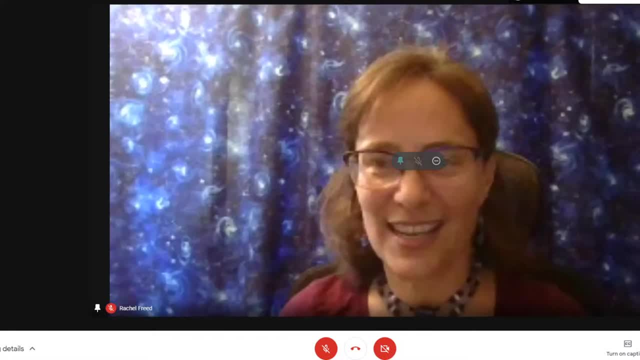 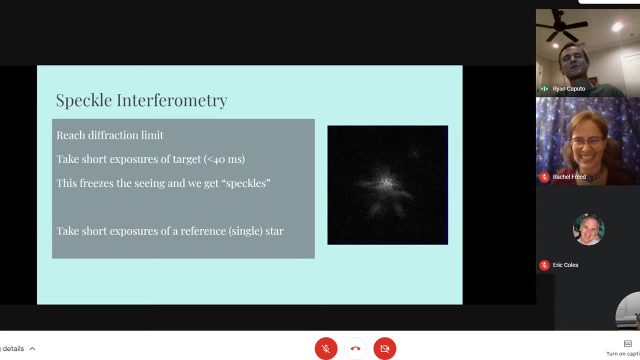 but the I guess the theme as each project goes along- I've done a few now- is I always want to do more. I can't just settle for doing the same thing over and over again. so I think, like the first project I did, I measured like one double star and I was like, oh yeah, I've measured one. 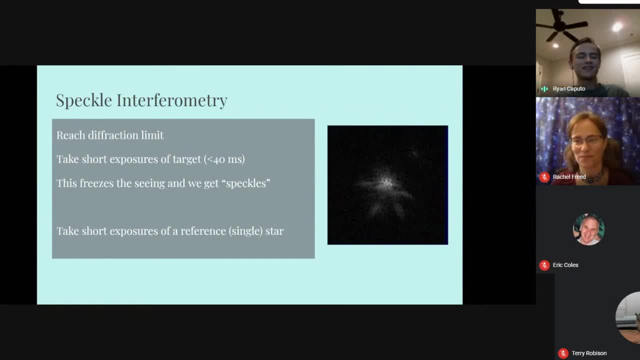 guys. and then the next project. I did like something around 12, and then I did faint and high delta magnitude, did it with Calla and now we're doing measurements below the seeing limit and the way we can push past this seeing limit, this five arc second limit, is by doing speckle. 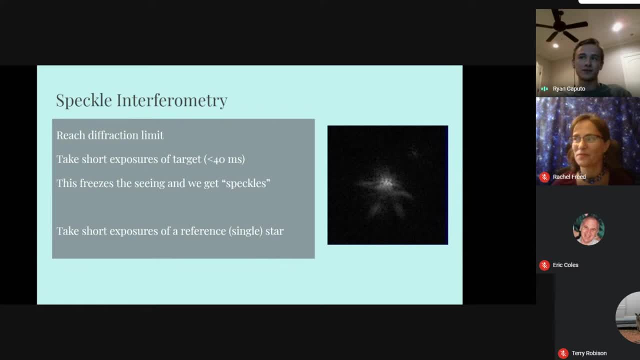 interferometry and it reaches the diffraction limit of a telescope. and the way it works is you take really short exposures of the target, Less than 40 milliseconds, and what this does is it freezes the scene and the specific- I wouldn't say aberrations, but I guess distortions might be a better word- The specific. 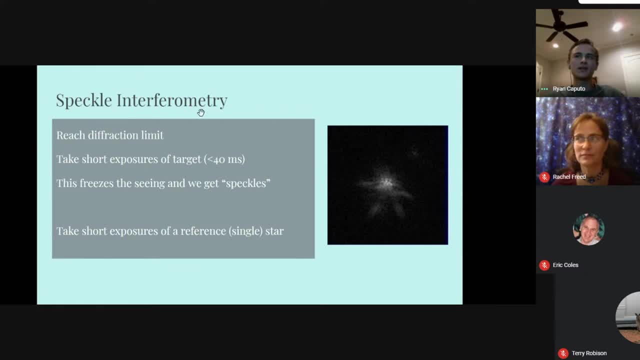 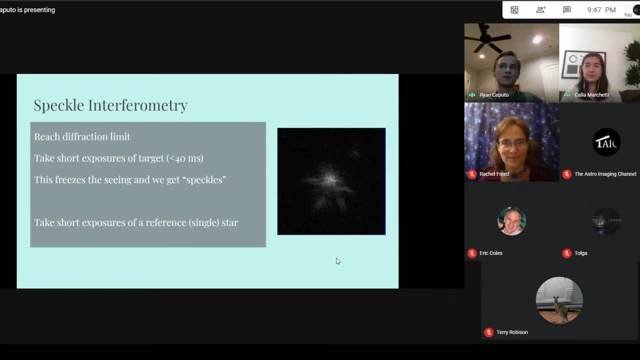 distortions that the atmosphere causes is it breaks the image up into a pattern of speckles, and these speckles, the key to these speckles, is that they're diffraction limited. They're technically diffraction limited images because if the scene were to destroy, 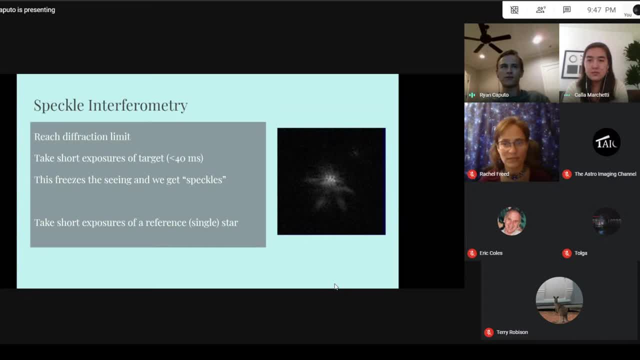 the image. we could never recover that information because we can't recover information that's lost. The information's technically still there. so in this image on the right you see a bunch of dots. This is of two stars. The information of those two stars. 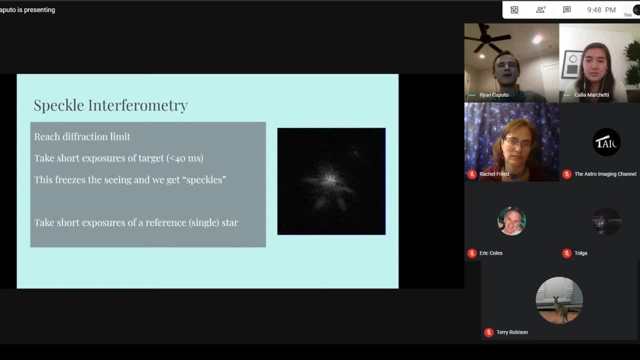 is still contained within that frame. It's just scrambled up, and the specific way it's scrambled is these speckles, these diffraction limited speckles, are superimposed on top of each other and there's like a lot of speckles. I'm not sure if you can see it, but there's a lot of speckles. 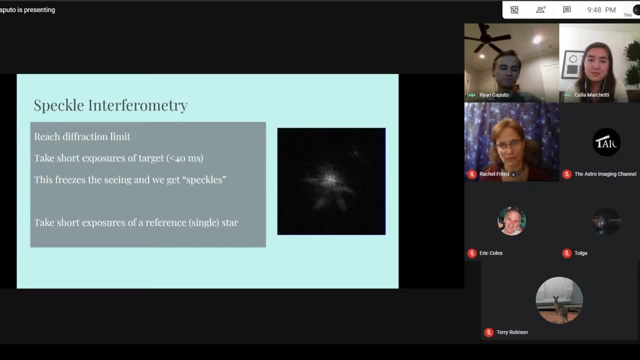 and I'm not sure how many, but this was taken with the Mount Wilson telescope, the 60-inch, so I mean you can visually see perhaps nine or ten or so, but there's probably 50 or 100 speckles in. 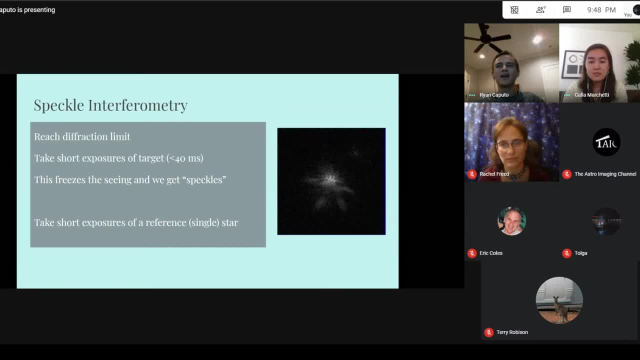 there, all superimposed, all mashed together, and each one of those is diffraction limited, and if we can somehow get that information out, then we can reach the diffraction limit, and so this is distinct from lucky imaging. It's a different way to reach the diffraction limit. 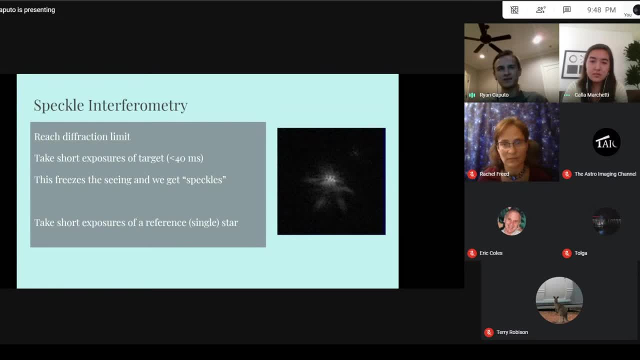 It's a bit more suited for double-scrolling. And then, as a side note, we also take short exposures of a reference star, which is any star, that's a single star and not a double, and that allows us to clean up some of the aberrations, like, for example, if the collimation's off, or just in general. 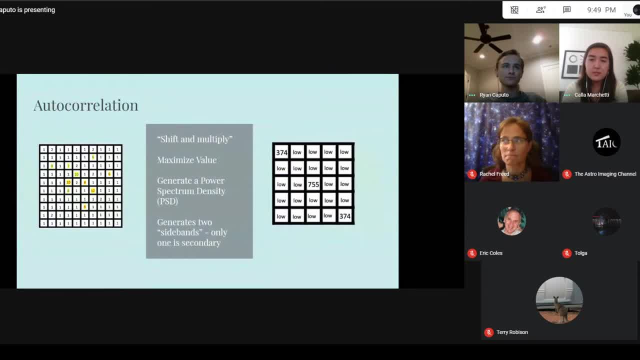 it improves the visibility somewhat, And so every double star image has many speckles, with both the primary and the secondary, and you can see in the figure on the left there are the brightness of the primaries, are the red numbers and then the brightness of the secondaries. 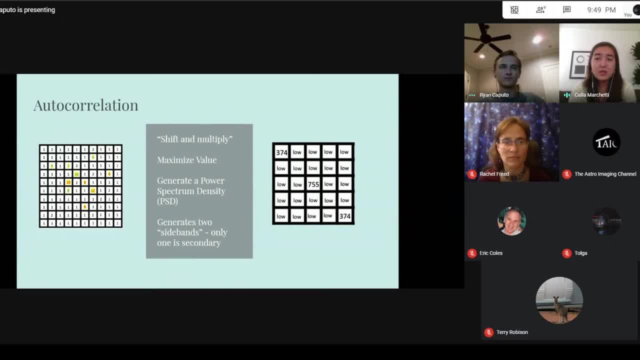 are up two and two to the left from their corresponding primaries, and those are the numbers in green, And this, of course, is a simplified picture of what a double star image looks like. A real double star image has a grid that's much bigger than 10 by 10.. 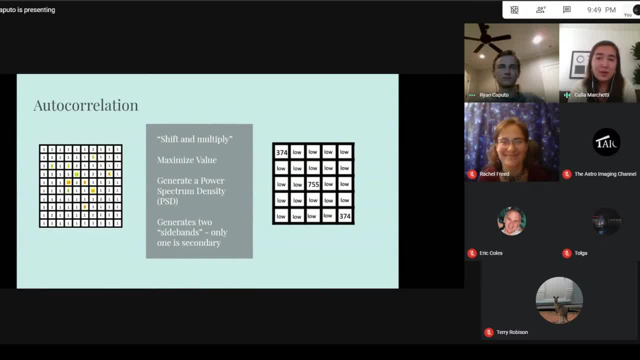 There's a lot more than five speckles, and the brightness of a star takes up more than one pixel. but this grid is a good representation to show what autocorrelation does, and in autocorrelation a copy of this grid is made. 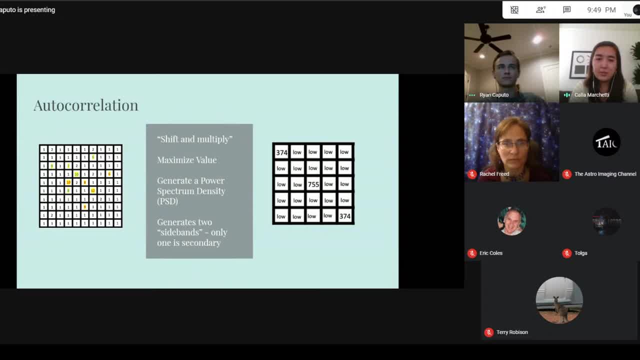 and it's moved in every direction on top of the original, And for each direction that the copy is moved, the brightnesses of the pixels are multiplied together and then all of these products are added together And depending on which direction the copy is shifted, the sum of the brightness products will vary in value. 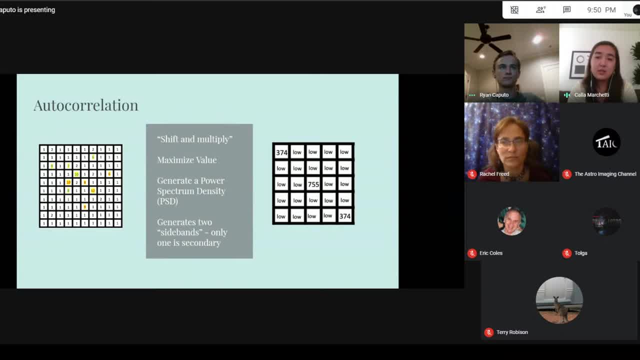 And so if the copy isn't shifted at all, the brightness of all the pixels will be multiplied by themselves and this will produce a large sum, and that is like the 755.. When you're on the right, And other large sums will be when the copy is shifted up. two and to the left, because that's when the primary 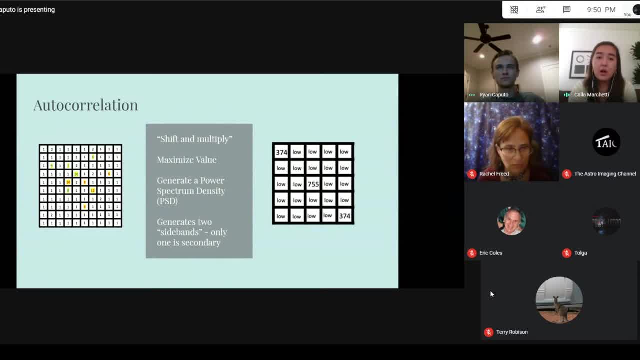 brightness is multiplied by the secondary's brightness, and also, when the copy is shifted, two to the right and two down, And that produces the same number. and this figure on the right is not an image, but it's a power spectrum density and it represents the brightnesses of the stars. but you can't actually do photometry on this. 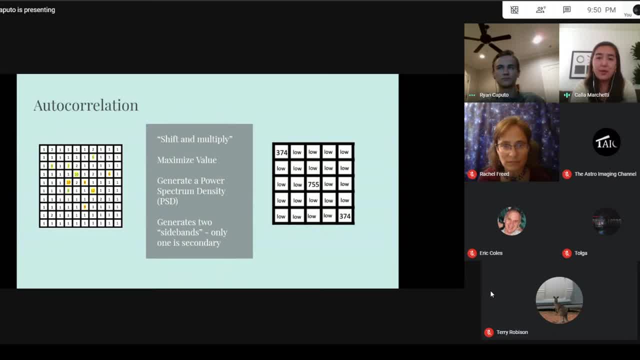 And It being a power of spectrum density is also shown by the two sidebands, which are the 374 values. Only one of those is the secondary, but because of the symmetry in shifting up and to the left versus down and to the right, there's a mirror image. 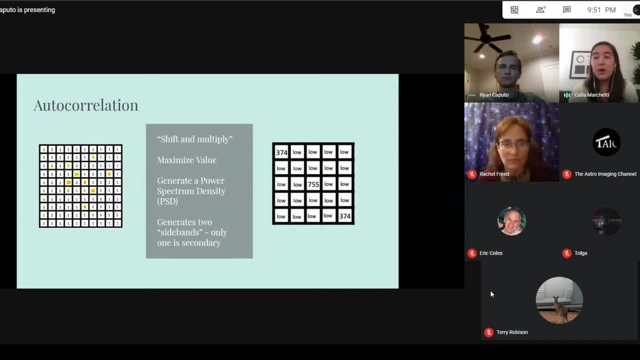 And so autocorrelation only works if you have a ballpark idea of where the secondary should be, so that you can pick between the two sidebands, And it doesn't work if you are discovering the double star. There needs to be previous measurements. But if you do have that previous measurement you can pick the correct sideband and measure the position, angle and separation. 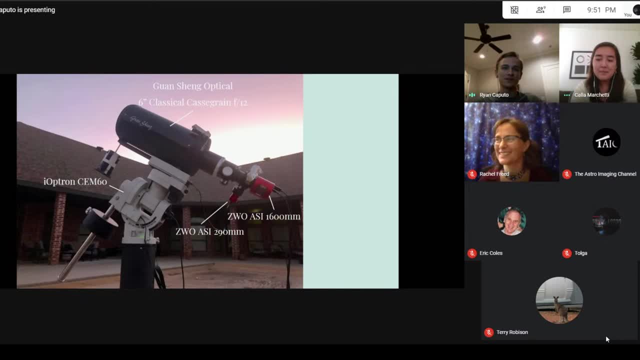 Okay, so this is the telescope that was used for this study And this is my telescope in the aptly named Purple Sky Observatory. I named it that because of the beautiful purple skies that sometimes are in the morning And I have the Guangxian Optical 6-inch Classical Castigrain. 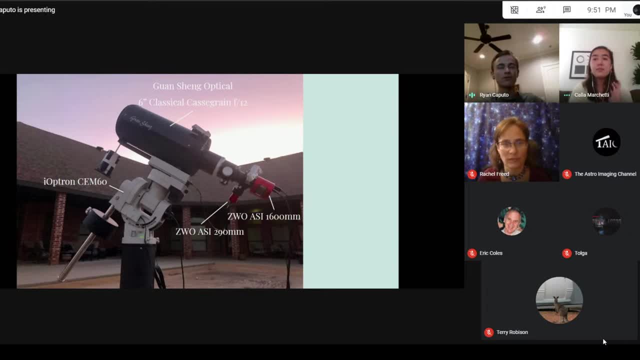 This operates at F12, and that's native. There's no focal reducers or extenders, And the Ioptron CE-M60,. this mount is a wonderful mount. I get amazing tracking with it And perhaps most importantly is the camera for Speckle at least. 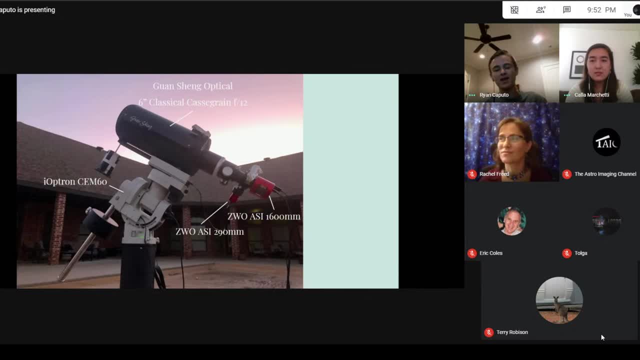 And this is the ZWO-ASI1600.. That camera, I'm sure, as many of you know, is the workhorse of amateur astrophotography, But in addition to astrophotography, it's an amazing camera for Speckle. 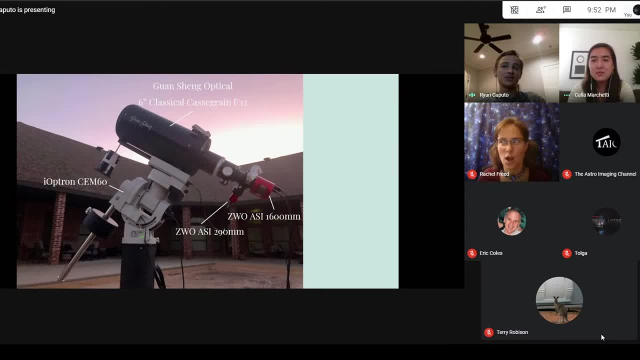 There's a pretty big difference. There's a pretty big debate between whether CMOS or CCD chips are better, But for Speckle CMOS chips are vastly superior And that's because they have low read noise. The exposure times in Speckle are no greater than 40 milliseconds. 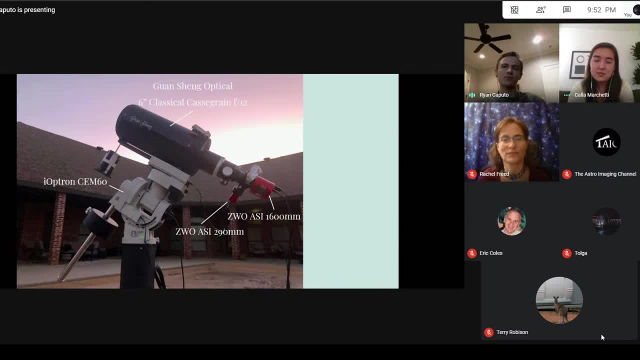 So we're automatically using just the very bottom of the full well of these pixels And that means that we need that bottom of the full well to have as little noise as possible, And that means we need to have the read noise To be as low as possible. 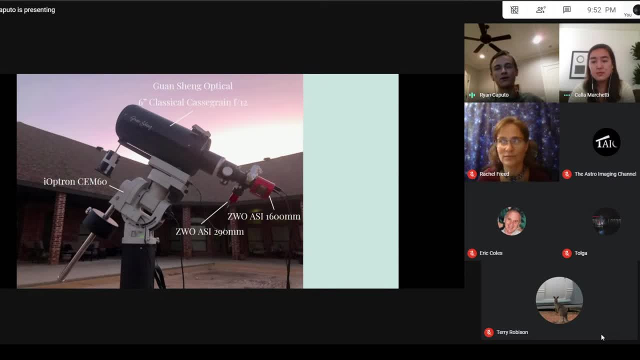 So we need a camera that can operate in a very high gain, low read noise operation, And the CMOS chips are very well suited for this task. In addition, CCD chips take on the order of about a second to read out, Whereas CMOS chips are faster, a lot faster. 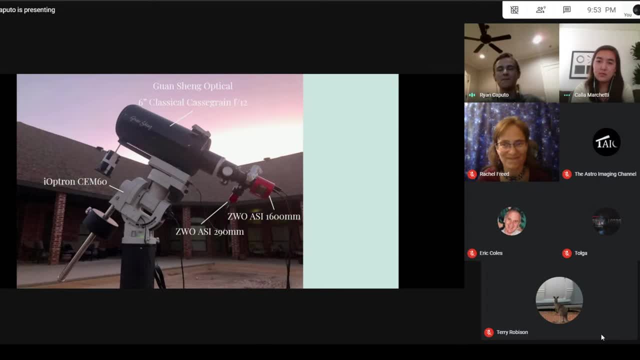 Perhaps you know 5-10 milliseconds to read out Callan and I usually take around 4,000 pictures per second For a double star somewhere around there, Because you have to take pictures for the target star as well as the reference star. 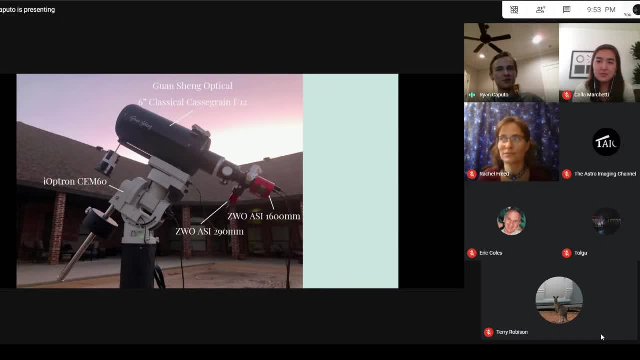 So I wouldn't really want to sit there for over an hour waiting for images to download. That would have a very low duty cycle, And so the CMOS chips are pretty much only suitable, Or Speckle interferometry can only be done on CMOS chips. 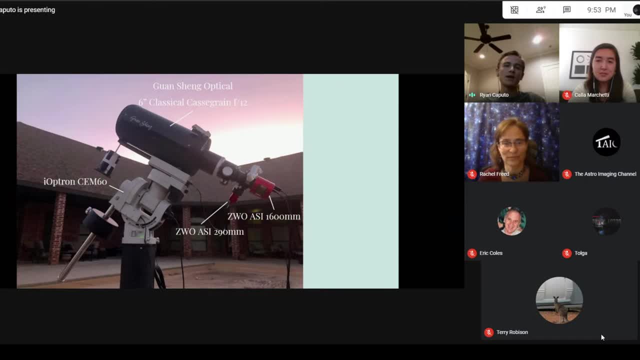 Doing it on CCD is very difficult, And I also have the ASI 290 for guiding, Although you don't need to guide with Speckle interferometry Because, since you're taking short exposures, the tracking doesn't really matter. However, or actually, this is really good. 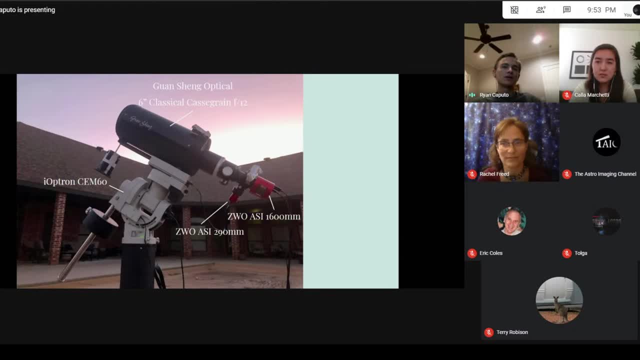 Because it's like planetary imaging, Where the only thing that matters is the telescope, And as long as your mount can point somewhere And not move off, not have random arc minute size jumps, Then you're able to take science data, And so it really kind of opens the door to a lot of people. 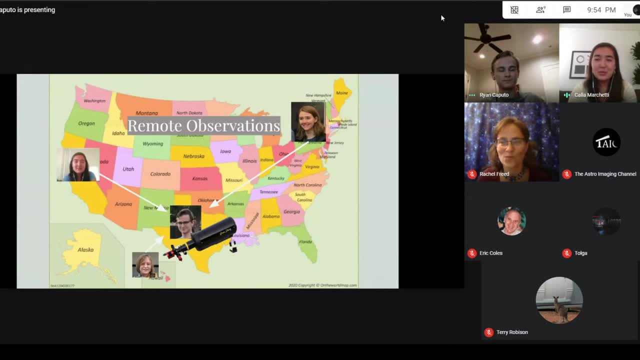 And so I don't have a telescope. And yet I was able to use Ryan's telescope to do this Speckle interferometry. But Ryan lives about a thousand miles away from me So I had to use his telescope remotely. So I use any desk to log into Ryan's desktop. 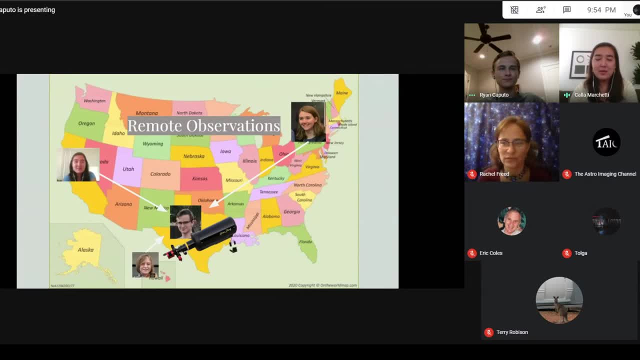 So on my screen I see Ryan's screen And when I move my mouse it moves the mouse on his computer So I can use the software he has to control the telescope and take images. And we also had two other students joining us. 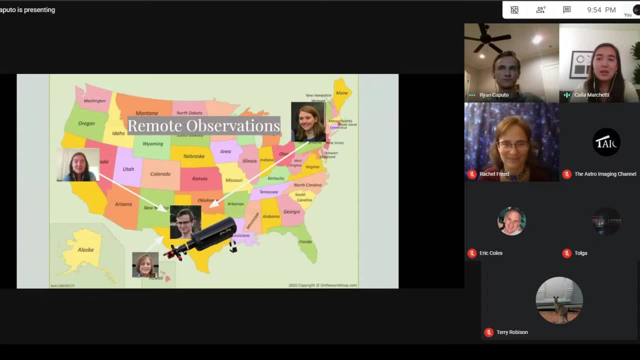 We had Jed and Jose. We had Jed in Hawaii, who was there for the beginning part, And Caroline in New York And she woke up really early to catch us at the end And Ryan and I observed the whole night. Ryan was there to make sure that we didn't break his telescope by slewing it into a wall. 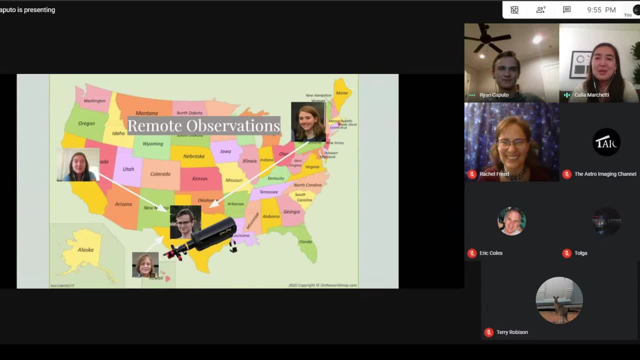 Or make sure the cables don't get tangled. And I was there because it was my first time ever controlling a telescope And it was really fun. But the idea with remote observation is that because students from different time zones can all participate and work with one telescope, 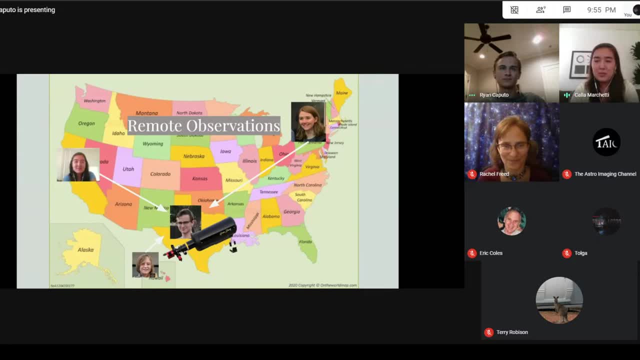 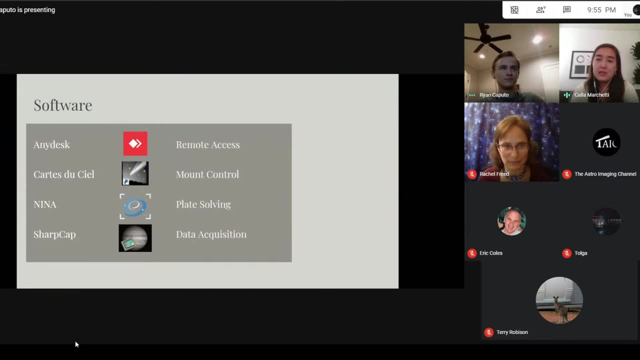 you don't need to stay up all night to get a full night of observing, And so we used for this observation. we used any desk to remotely log into Ryan's desktop. We used cars to seal as mount control and to slew to our targets. 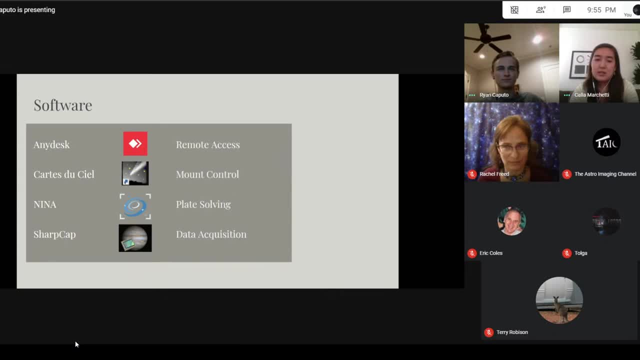 And we used Nina for plate solving and SharpCap to center the images and to change exposure time and to take the captures. And we chose these programs because they're free, but also because they're pretty user friendly, especially for someone like myself who has no prior knowledge about telescopes. 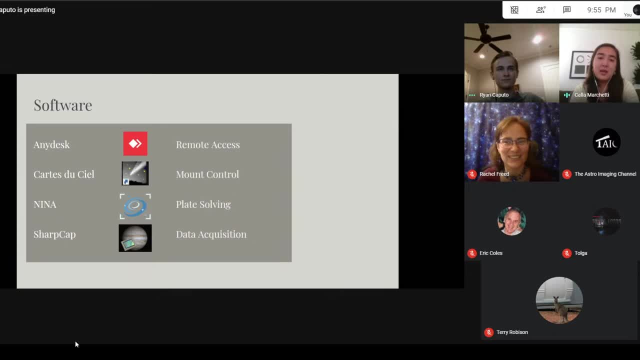 The first night we did it. a lot of time was spent getting to know the programs and triple checking before every button was clicked And we got 10 stars that night. But by the second night I had my bearings a lot better with the programs. 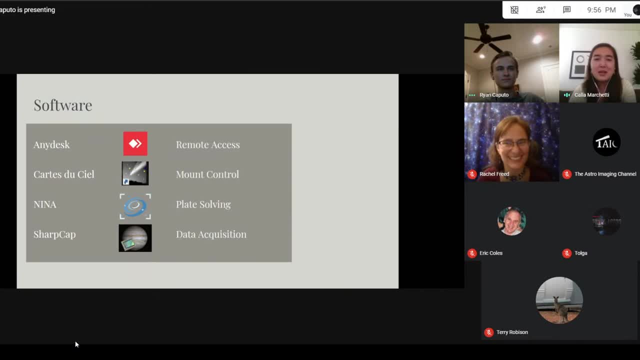 And we got 31.. And we got 31 double stars. So that's a steep learning curve, I guess. And I want to say that Calla was, you know, chilling in her house, nice and warm, while I was outside sweating in the Texas heat covering bugs for seven hours straight. 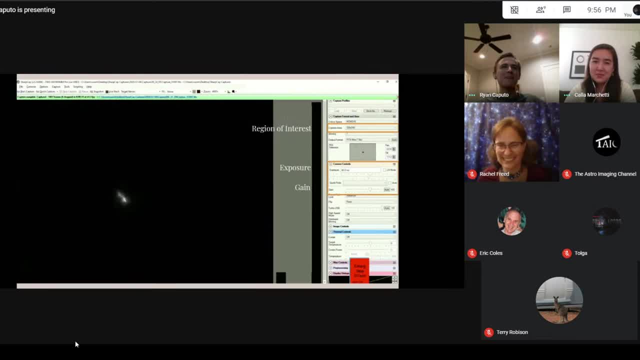 So a big difference in what we were actually doing. This is SharpCap in action And you can see the most prominent thing is a double star in the middle, And this was actually taken with Russ Jenae. He has an observatory And I'll talk about that later, but his observatory is doing speckle. 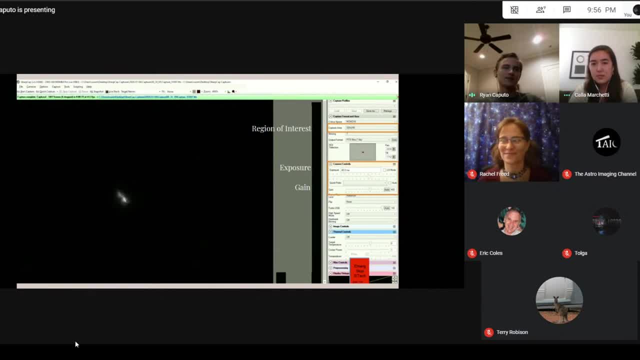 And Calla took this picture of any desk which is screen sharing Russ's observatory computer. So this is on Russ's computer, but Calla took the screenshot, So I think that's pretty cool And this double star is somewhere around three arc seconds. 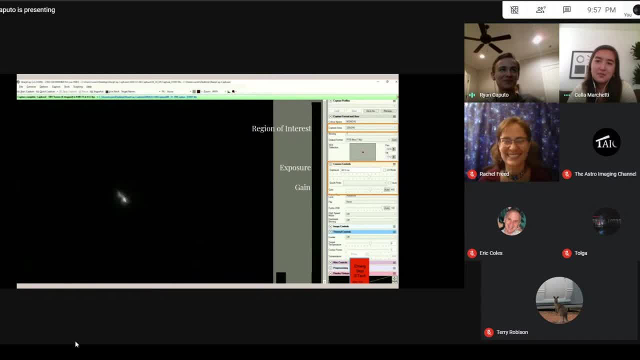 I'm not sure which one. There's a lot. They get jumbled around. But if this were doing, if we were doing a traditional CCD imaging technique, this star like I would look at this picture and be like that's not going to work. 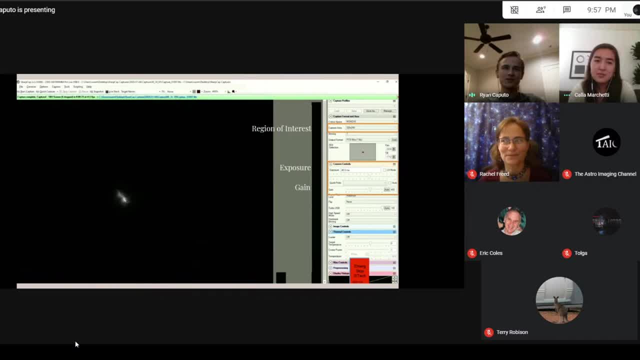 Because you can see, it's smeared. There's not a clear separation. There's no, they're not round. However, for speckle, this is actually a wide pair, Because speckle can reach the diffraction limit regardless of the scene. 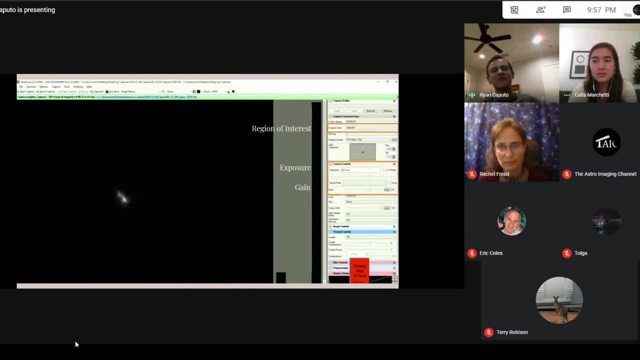 Relatively regardless of the scene And maybe if you have like 10 arc seconds full and half maximum, you might want to close up for the night. But in average scene conditions it can reach the diffraction limit And Russ has an 11-inch telescope. 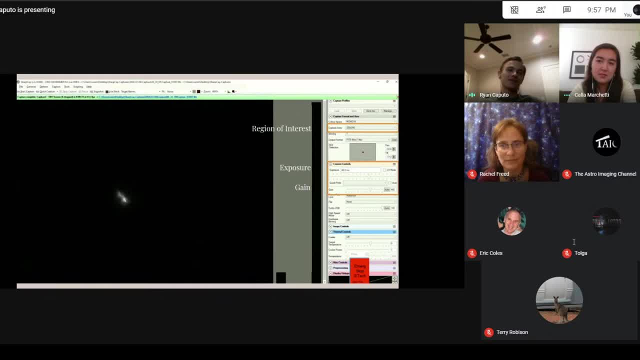 So three arc seconds is nothing for that, And we, Calla and I, have image targets where we look at it and it's a star. It's like that is a single star. There's no way There's a double star in there. 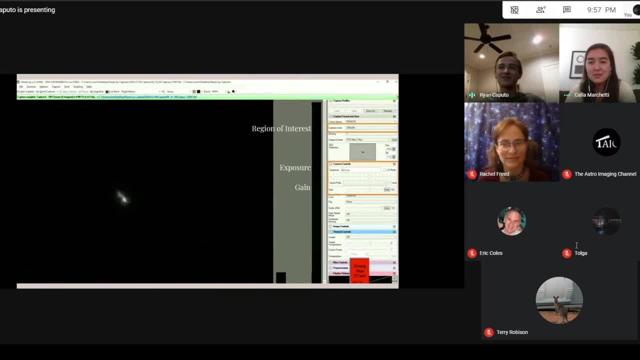 And then we'll do the reduction and out pops two stars just like magic. So this is, believe it or not, a wide pair for speckle. The things to look at is the region of interest up on the right. That is really important because the 1600 produces it's 32 megabytes per frame. 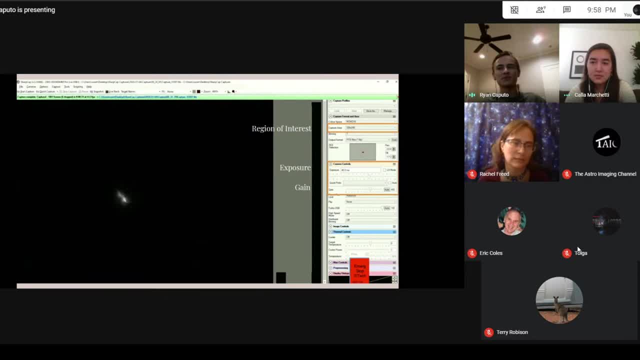 And if you're doing 20 frames per second, that's a lot of data per second that you're going to be collecting And you don't need that. And so the region of interest is very important, And for planetary astrophotography it's essentially the same region of interest. 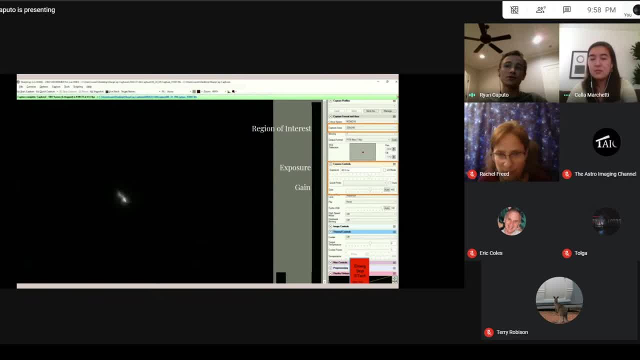 And then the exposure time and gain. usually exposure is at 40 milliseconds because not every star is sixth magnitude. There's more seventh magnitude than sixth and more eighth than seventh. So most targets are going to be fainter And so 40 milliseconds gets as much light as possible. 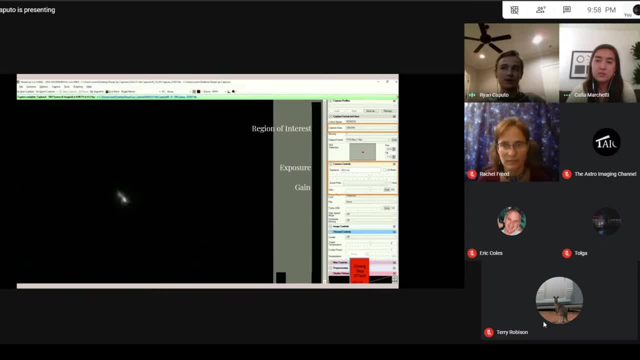 And the gain is always over 200, because a low gain has higher read noise And even though a high gain looks like the image is more noisy, it's just because it's doing well, it's doing two things. It's doing a stretch of the image in the camera at least. 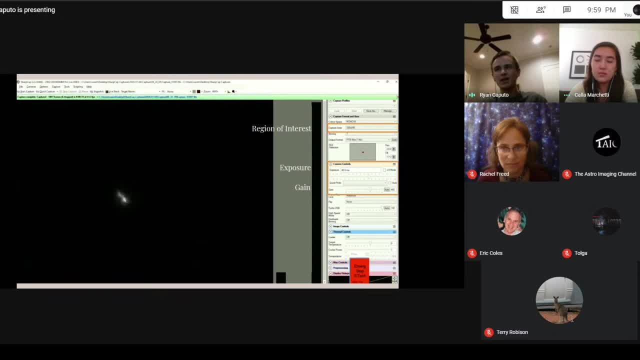 And then it's also changing the read characteristics And it actually lowers or increases the signal to noise, even though it appears to make the image more noisy. And the point at which you really need to hit is a gain of 200, at least for the 1600 chip. 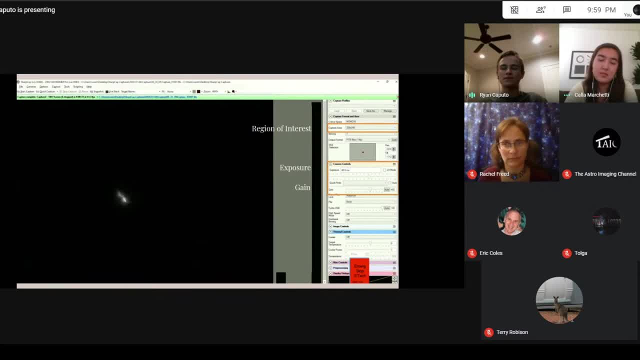 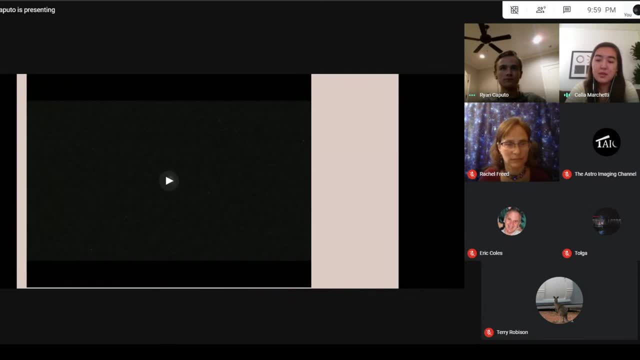 Anything over 200, and you are pretty much at about as low of read noise as you're going to get, And you're in really good territory for that. And so this is what a speckle capture looks like. These are 40 millisecond exposures of a 1.89 arc. second separation: double. 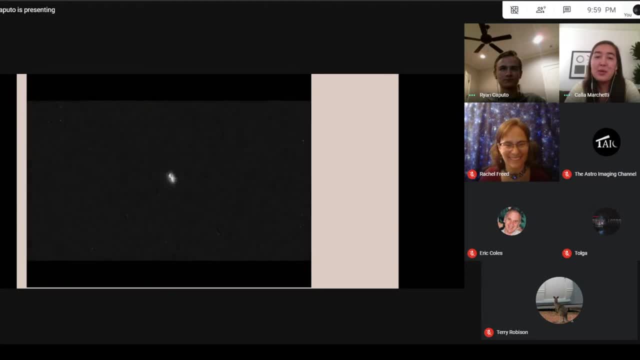 And we were really excited to get this star because we thought that two arc seconds of separation was going to be the limit of Orion's telescope. So getting under two and under 1.9 was very exciting. And we actually had to image this star twice because I was impatient and I wanted to image it before it was high enough in the sky. 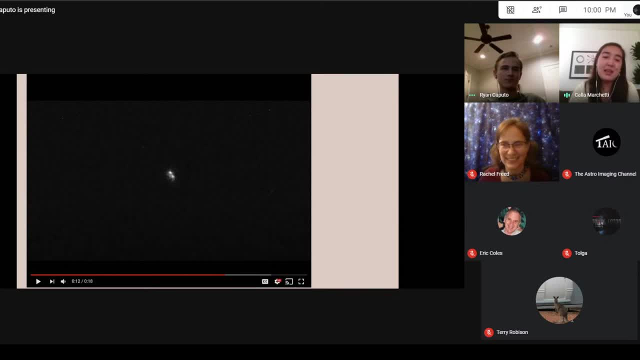 And then the images were bad. But you can see that in that video the stars were jumping around a lot And the noise from the atmosphere varied from frame to frame. But when you process the image using autocorrelation, a lot of this noise goes away. 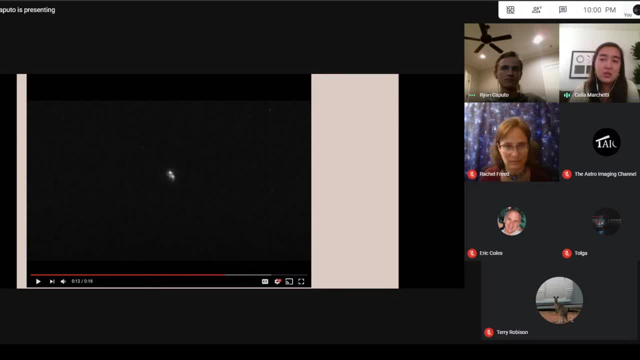 And in that video you can also see that- the stars. you can see that there's two stars there And that's because the seeing happened to be bad. It was very good that night And, like Ryan was saying in the past slide, most of the time stars look like a single blob. 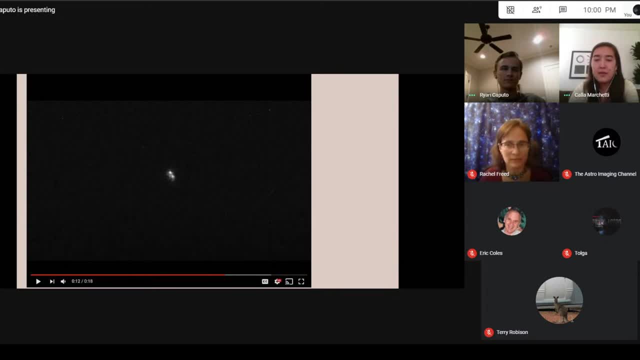 And you have to process them in order to see that there's two stars there. And one thing you might be wondering is: why can't we just do a short exposure like this and then measure, just like a traditional CCD technique, where we go to some program and just set an aperture size and then just measure across and there we go. 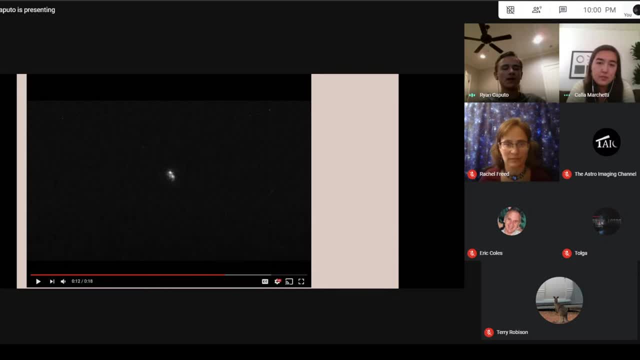 Because you can see two peaks there And they do look relatively well resolved. However, if you look at the image, you can see that there's two peaks there. However, if you look at the frames- and some frames are worse than others- the stars are oftentimes not round. 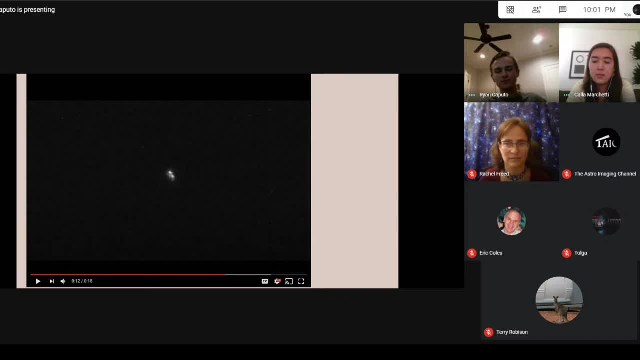 And that's because it's not the amount of tracking, It's just the atmosphere might blow one way, blow another way, And that makes the stars asymmetric. And so it's essentially the same rule in traditional CCD imaging Or, I guess, in any astrophotography or astroimaging. 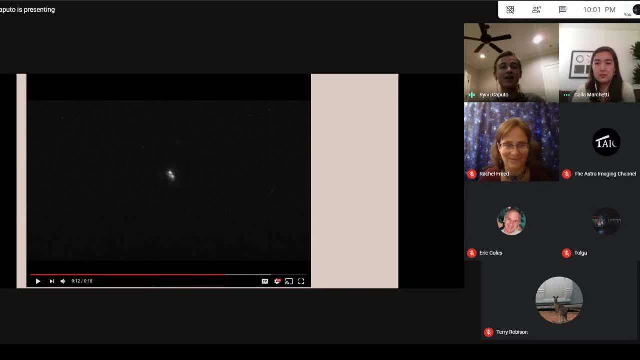 If your stars aren't round, you're doing something wrong. And in the case of speckle, we can't get round stars because the atmosphere is constantly moving And, at the pixel scales that we're operating at, you're never going to have round stars, unless you're in space, which we're not. 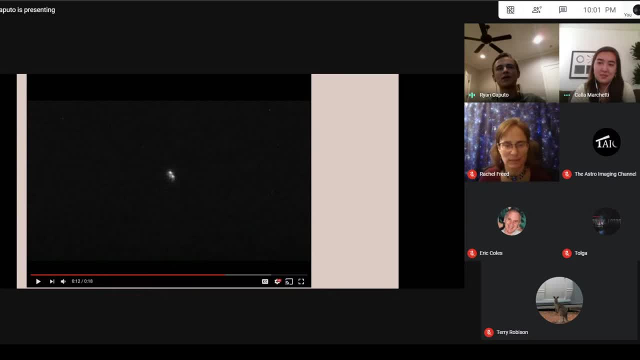 So speckle works well for even these stars that are partially resolved, like this one. And another thing to note is this was with the six-inch telescope and the Guangchian optical telescope, And it is 1.89 arc seconds, which is a lot. 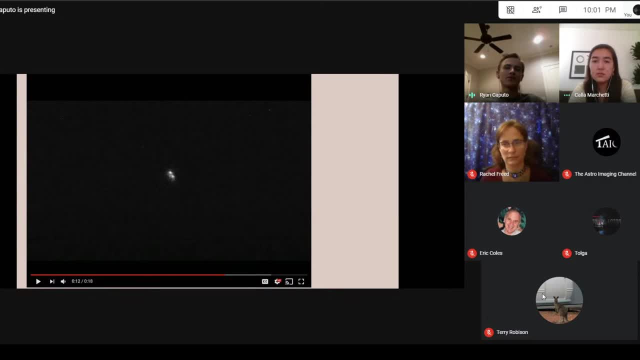 It's closer than we expected to be the limit I mentioned earlier that we could reach the diffraction limit, which for a six-inch should be about one arc. second, because I was in V band. Well, that assumes that the pixel scale is up to the task of that. 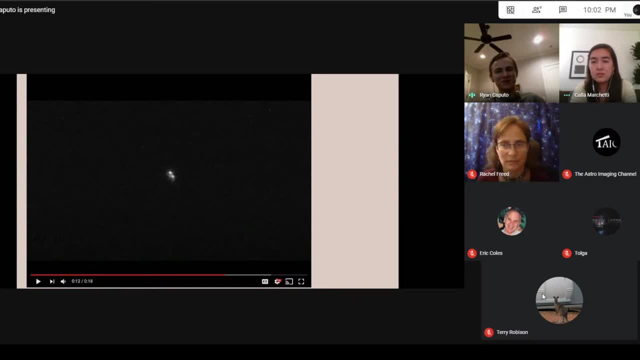 I'm operating at f12, which might be slow for some, but for speckle it's actually very fast. It's actually too fast. It's undersampled. It's optimal to have about seven to eight pixels across the ARRI disk. 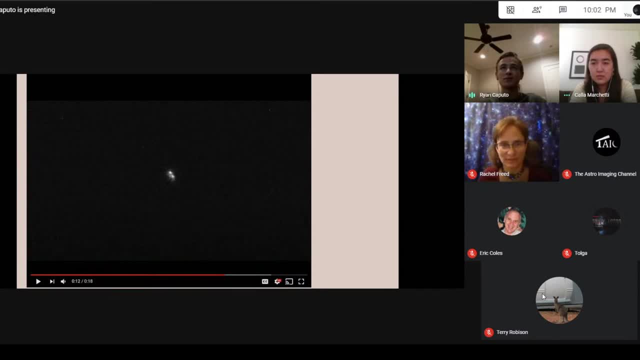 So seven to eight pixels across one arc second, so about 0.2 arc seconds per pixel. I have five pixels across the ARRI disk- 0.43 arc seconds per pixel, which is not enough pixels to reach the diffraction limit, because there's simply not enough. 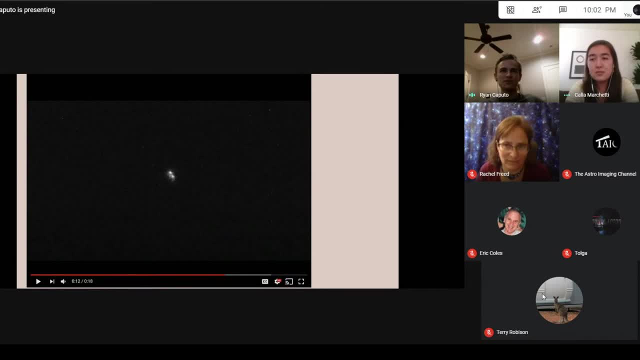 If there were two stars separated by an arc. second, there's just not enough pixels between those centroids or between the peaks To actually measure anything with confidence. About five pixels is the limit to what you can measure, regardless of the telescope aperture, which is what we found here. 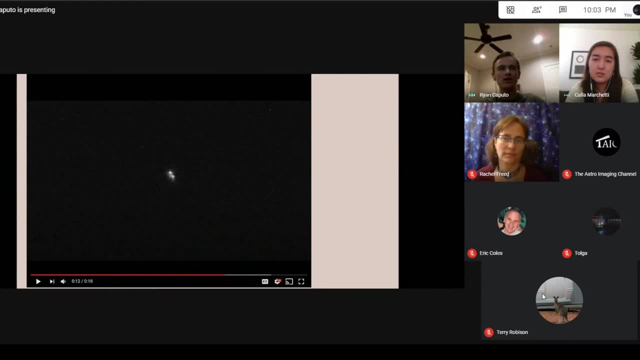 I think this is about 4.6 pixel separation, And this isn't totally bad though, because operating at f12, which is fast, is a benefit, because it is faster than something like f15 or f20. And it allows a little bit fainter stars to be measured. 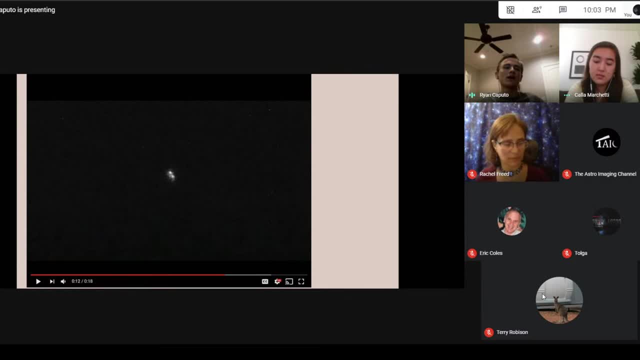 Because you're just packing more light into each pixel And we found experimentally that 10.3 was getting pretty faint. You could barely see a 10.3 star with a 40 millisecond exposure. So we suspect that somewhere between 10.5 and 11 is the faintest we could go, which is pretty good considering a six-inch aperture and 40 millisecond exposures. 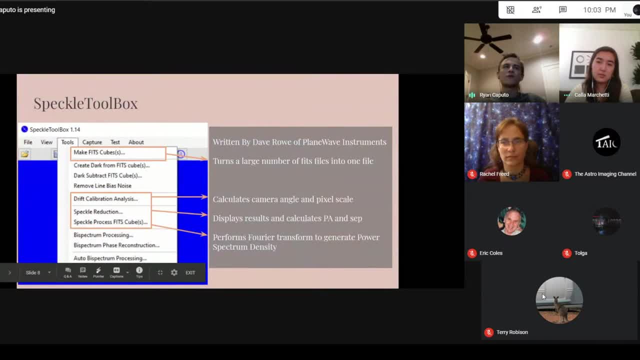 And the actual software that does the speckle reduction Is speckle toolbox And it's written by Dave Rowe of plane wave instruments. Many of you probably know his name. He is an amazing astronomer that has done so much for the amateur and professional astronomy community. 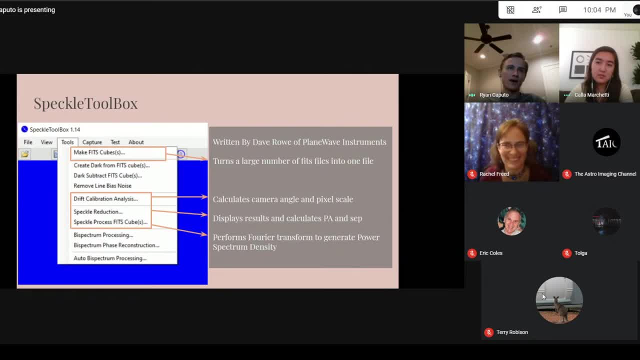 And one of those things is writing this amazing software that I don't know is if it's replicated. This is the only software I know that does speckle, Although I might be wrong. The first step is to make fits cubes. This turns the 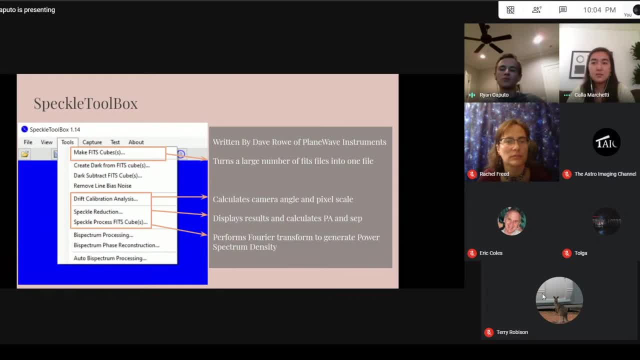 Giant image, pile the 500 frames or so of your target into one file, So it just puts them in a stack. It doesn't stack them like astrophotography stacking, It just puts them in a pile. So when you move the one file, it contains all the 500. 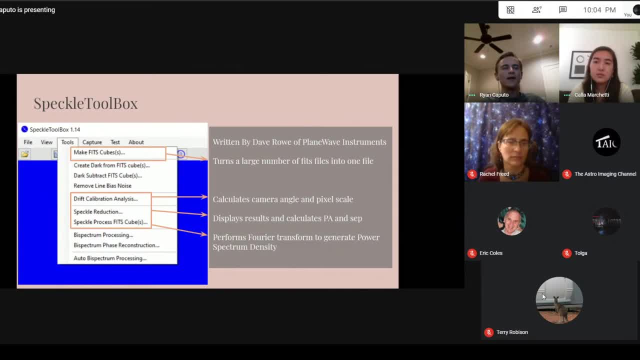 So you don't have to deal with a giant folder files, which is nice, And then we do. speckle process fits cubes, which performs for a transform to generate the power spectrum density. This does the technique that Calla was describing earlier, with the autocorrelation where it looks at the speckle. 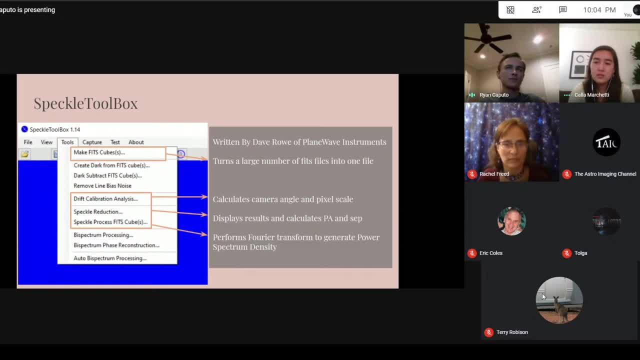 And it tries to match the primary speckle with the secondary speckle and figure out which speckle goes with which other speckle, And then the speckle reduction simply displays the PSD And then from that calculates the PA and SEP. 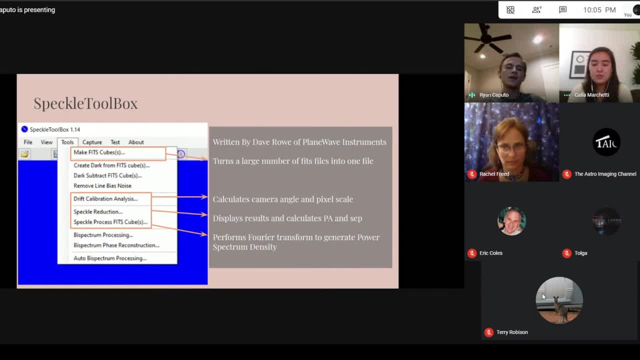 And it doesn't first calculate PA and SEP. It calculates the separation in pixels and then the orientation relative to the plate, So Like relative to a straight up on the image, The you have to supply it with the camera orientation and the pixel scale, which you can get one of two ways in the program. You can get it using a drift calibration, Which is a bit more complicated. You take a, you point towards a star, a single star, and then you turn off the tracking and take a sequence of images as the star drifts through the frame. 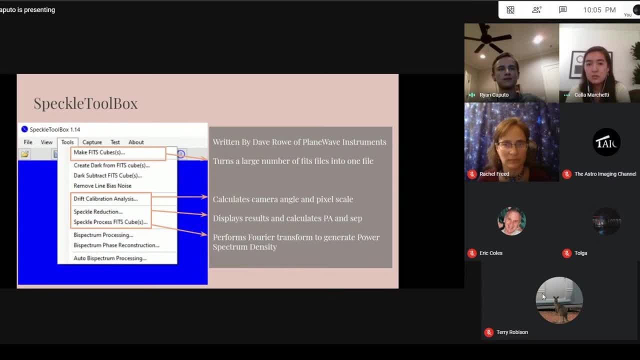 And you can put that into the program and it will automatically use the time codes that are in the image headers To find the rate at which it's moving, to calculate pixel scale, And then it can find the angle at which it's moving to find the camera angle. 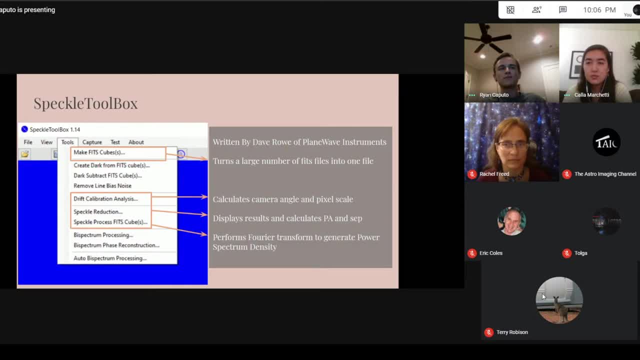 This is really useful because it replaces the option of plate solve. We are able to do plate solves because I can just turn off the region of interest, get the entire image chip And for me the field of view is like 23 by 30 arc minutes. 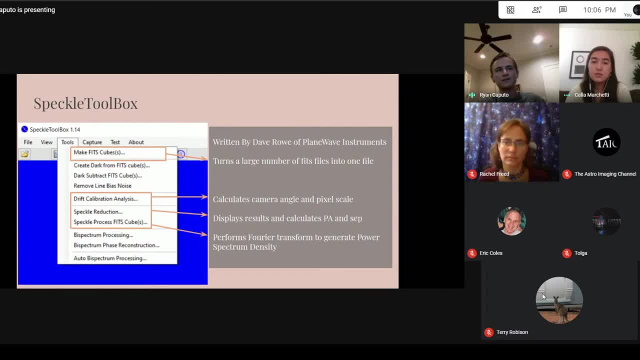 Somewhere around there. Okay, And that's more than enough for plate solving. We can get the camera angle and pixel scale from there, But some telescopes like? I know an astronomer, Rick Watson, who does speckle. he uses a 22-inch telescope. 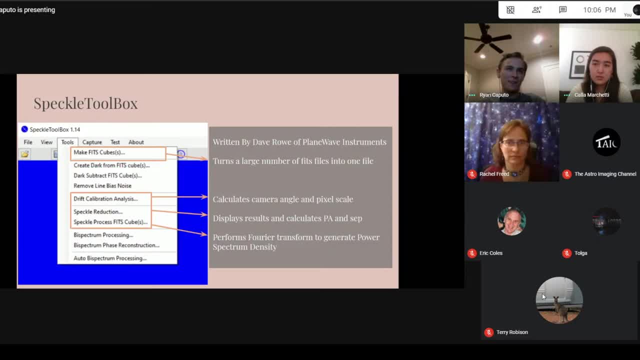 I believe F16 with the ASI 290.. Which is a super small chip And it has something like a two arc minute field of view And I don't think you're going to be plate solving a two arc minute field of view. 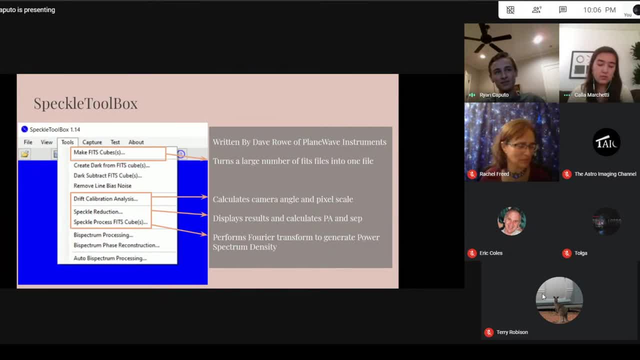 Unless you have some really special software. So the drift calibration works. if you can see a star, It only takes a single star to work, And if you can't do a drift calibration, it means you can't see any stars, And then while you're doing speckle, you can't see stars. 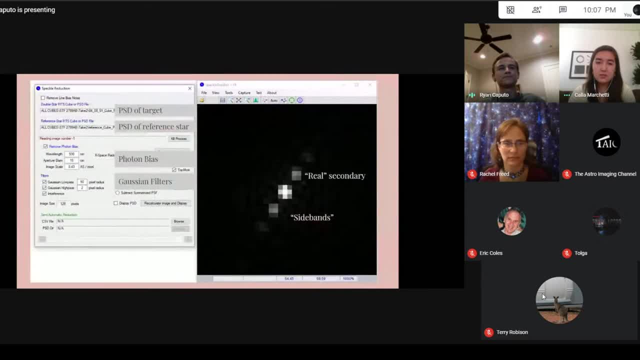 So a drift calibration is an amazing tool that always works, And this is what a speckle reduction looks like: You have a place to put the PSC of your target and the PSC of your reference, Which lowers the noise in the image because it repairs the atmosphere. 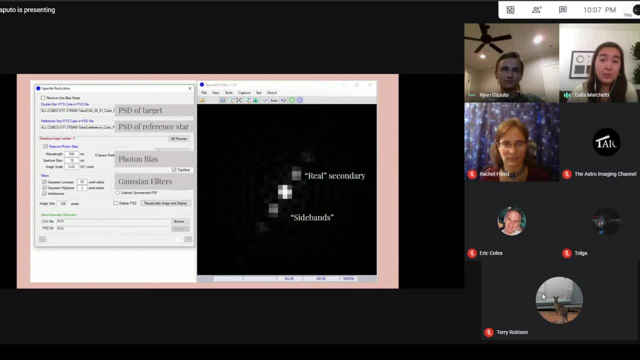 And then removing the photo- The photon bias further lessens the noise- And then changing the Gaussian filters will sharpen the image And then, once that's done, what's produced is the image on the right, Where you can see a bright primary and then two side bands. 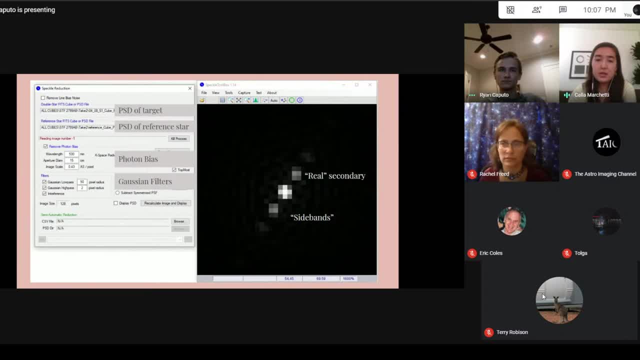 One of which is a secondary, And this is a pretty good image here. It's actually of the same 1.89 arc, second star from the video And you can see that this is a lot clearer, A lot less noise, And it's ready to image. 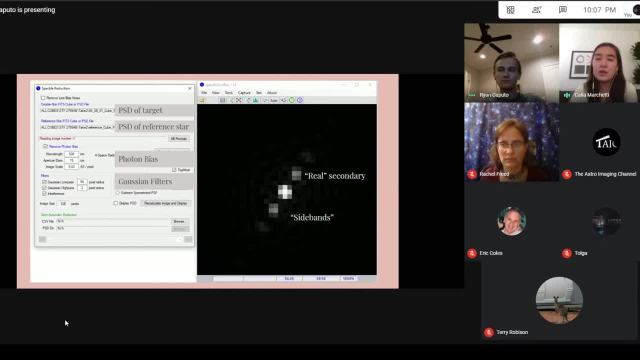 And because it's clear, you can probably get a pretty good measurement of the position angle separation. And one thing I want to quickly mention is that, even though this image here that we see in speckle toolbox is a completely fake image- It's an autocorrelation, not a real image. 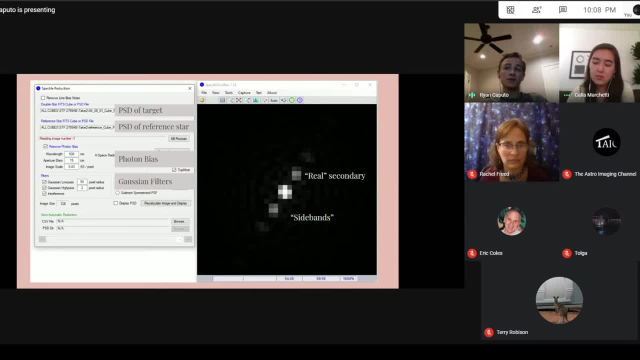 It still retains the same pixel scale and orientation as the real image. So if we measure the distance, the separation of pixels and the orientation, That matches to real life And that isn't broken. So we can use a real picture and then transfer that calibration data, the pixel scale and stuff, to the pseudo image. I guess. 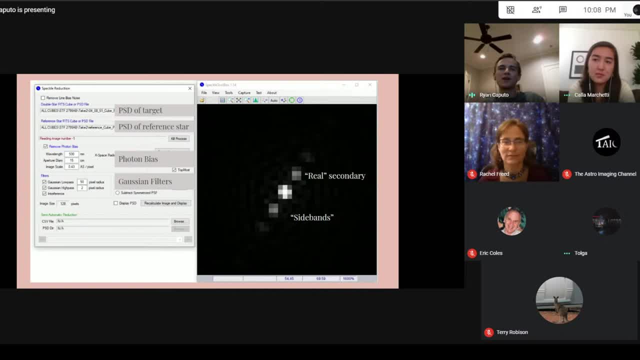 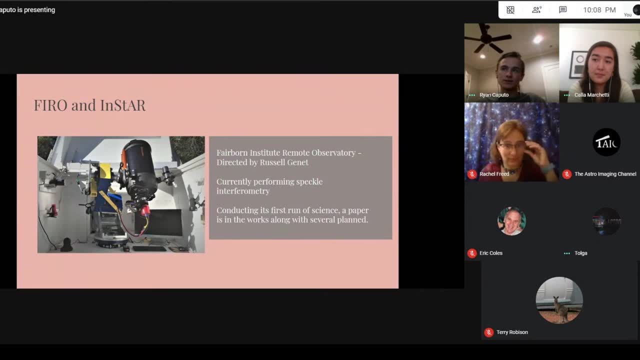 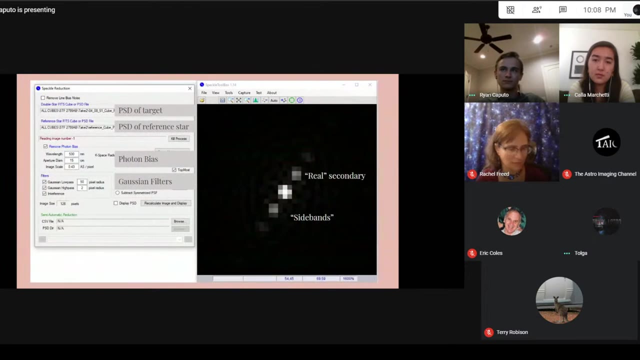 The fake image And it won't break anything, And that's how we're able to make these measurements easily. I have a question for you guys. Yes, So correct me if I'm wrong. I may be wrong about this, But if we look at those two side images, we don't know which one is the real star, right? 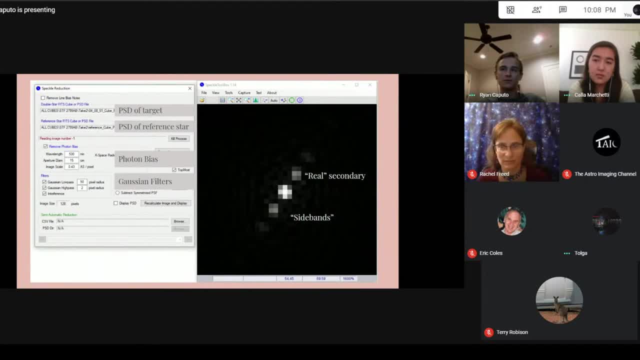 It could be either one or the other. Yes, It could be either one or the other, Right? So that's all I wanted to say. And, by the way, don't use that word fake. Okay, Actually, I got interrupted. 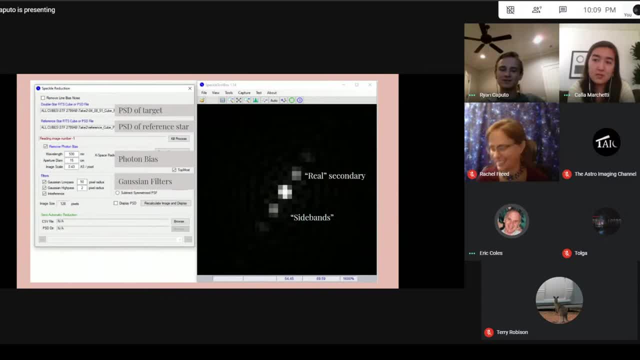 Could I ask you another question or two? Yes, So you showed us two partially resolved stars in one of the prior images. Yes, Are you going to show us the two stars resolved using speckle? This is those two stars resolved in speckle. 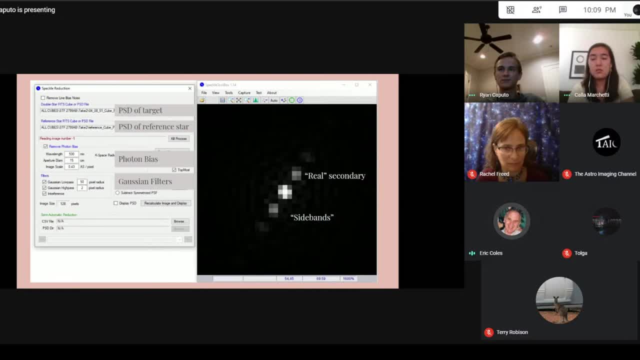 So one of those is a star and one of those is a sideband. Yes, This image is deceptive. It looks like a picture of the star, Like the bright spot in the middle That looks like the primary star. That's actually not a star. 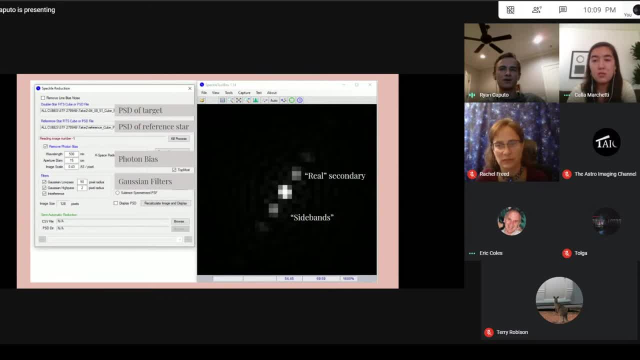 It is a representation of the star. It technically the very center pixel is technically, I believe, the image squared, If that makes any sense. It's a Fourier transform, So it doesn't have any resemblance or it doesn't have any correspondence to the real image, except for the pixel scale and orientation remaining the same. 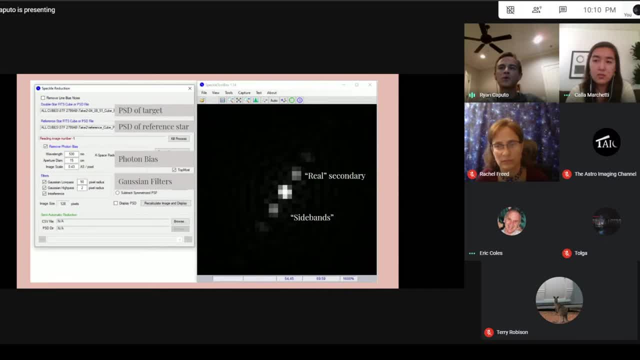 It is a representation of the image And that's why we have these two sidebands. So this is not a picture of the two stars in any way. Yes, This is absolutely not a picture of the two stars And it is deceptive. 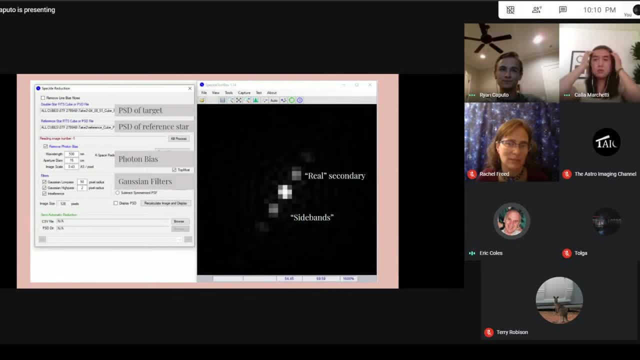 It really does look like it might be Right. It does, And so are we going to get to that point. or is that not the objective of your speckle analysis? That is not the objective, because we don't need to get to that point. 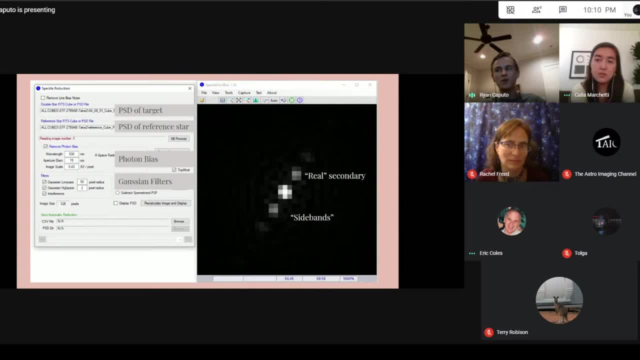 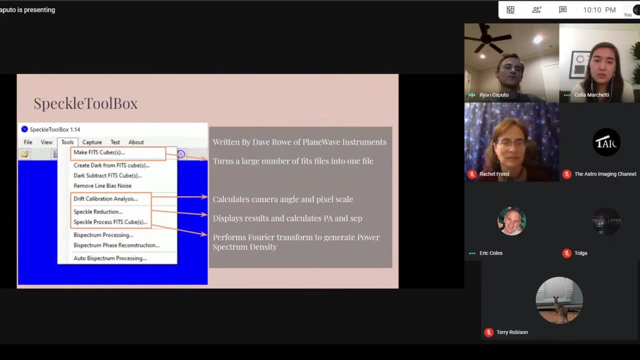 There is a way to get to that point where we can do bispectrum, which Dave Rowe also has. I can actually show you in the tools right below, speckle processes of bispectrum processing And this goes from: this does normal speckle but then it does some fancy under the hood stuff which I'm not sure how exactly works, but it it generates a diffraction limited image. 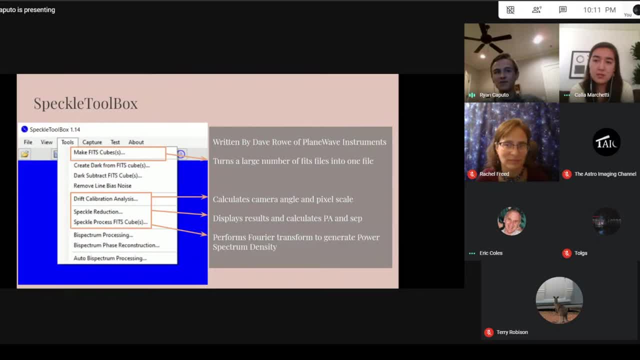 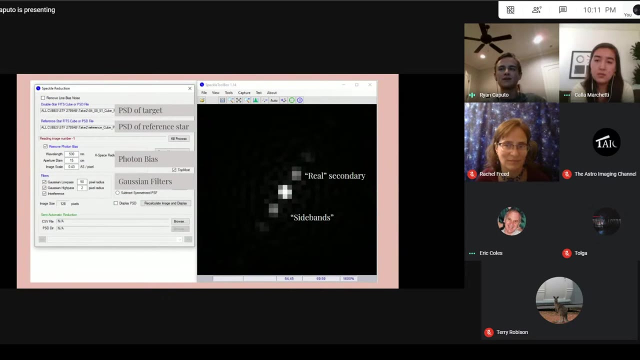 So not a diffraction, limited representation of an image, A real image that can have photometry done on it- And Calla and I are working to see how reliable that photometry is- But the speckle image that we get here. photometry cannot be done on this. 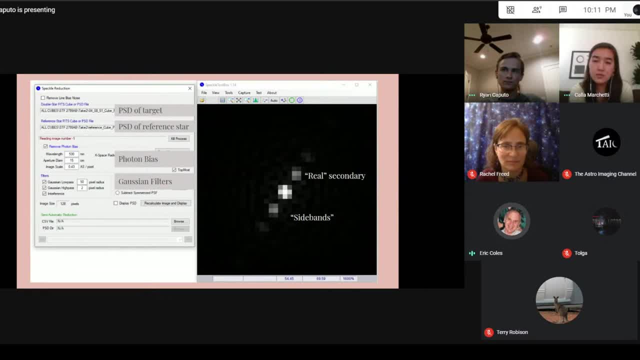 So I have another question: How does this compare to, say, lucky imaging, really zooming in and then doing an analysis with something like auto stacker And aligning All those 50 frames per second or 100 frames, whatever you're taking with your CMOS camera, the result of which will be an image of two stars as compared to what you're showing us here? 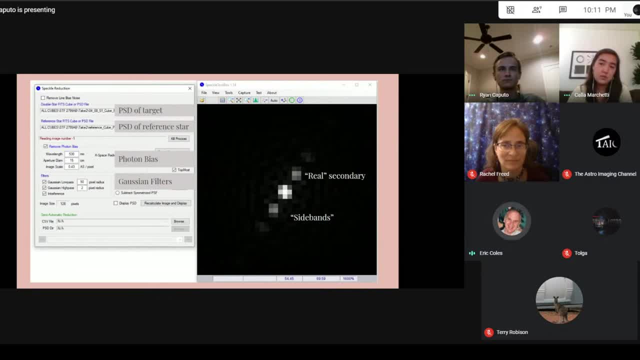 So if you took the same data and did an analysis by auto stacker, how would that compare to what you're doing? I have done auto stacker, I use Registax, but same in principle, So the images that it gives are clear and I have not done a study. 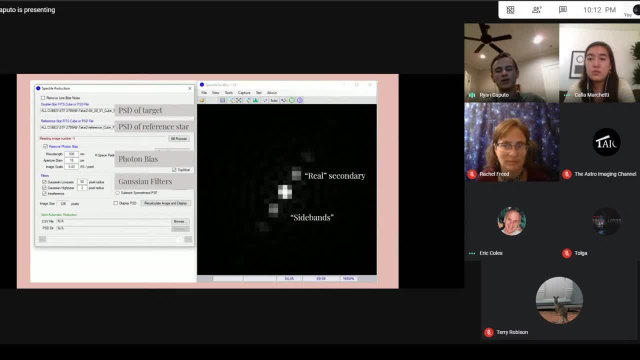 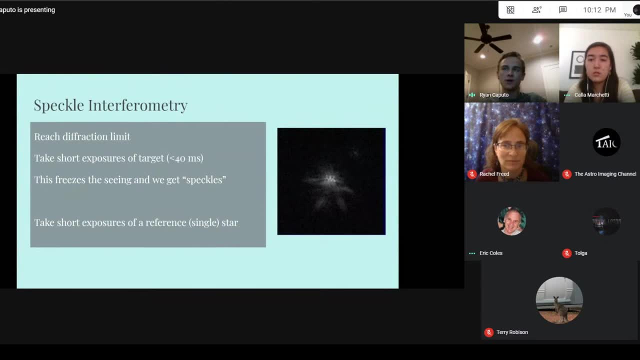 I don't know of any studies that have compared speckle to lucky imaging. However, if we look at this picture here, this was taken on a 1.5 meter telescope and lucky imaging depends on getting a good picture, So you have to get lucky in the name where? 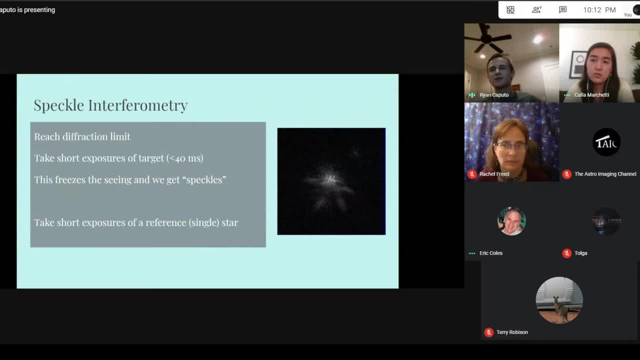 If you have a large aperture And you have very clear pixels that are over the aperture, that there's always going to be distortion and you're never going to get a lucky picture. I believe the probability of a lucky image drastically decreases as the aperture increases. 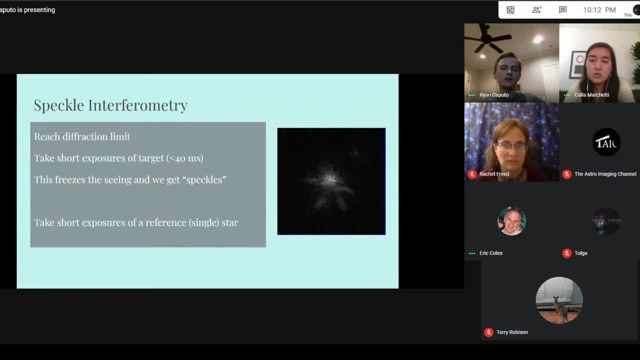 And so with the six inch telescope which is what I have, I would imagine that doing speckle and lucky imaging with auto stacker would probably give about the same results. But for a larger telescope, say in the range of A meter or so, anything above half a meter, you're going to get diminishing returns where you're going to need a lot of frames because there's very few lucky frames within that. 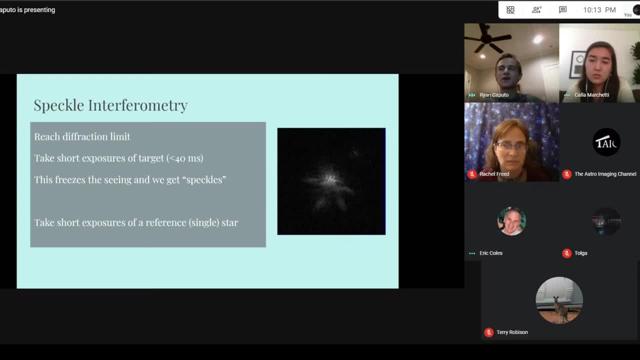 And you know, imagine if you were to stack this frame and frames similar to it over and over again. you wouldn't be able to resolve the two stars effectively. So speckled essentially works much farther than lucky imaging does. OK, thanks, 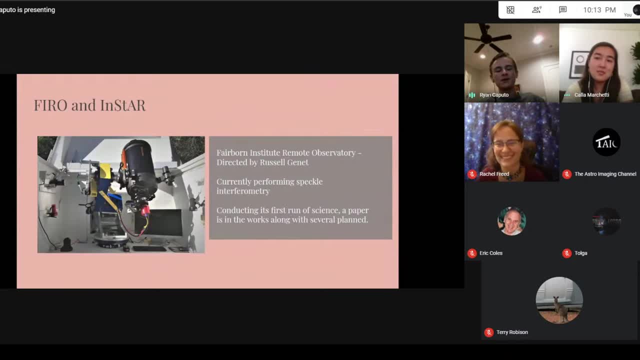 As we go forward, because again we have to do more each time. It's that, I guess, human pursuit. Rachel and Russ have been scheming to better manipulate us to do more research, And one way I guess that we're susceptible is doing 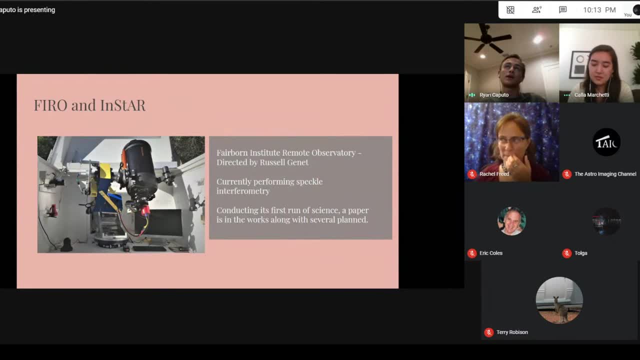 Rachel and Russ have created the in star student robotic telescope, Our student robotic telescope network, Which so far its primary goal is to do speckle interferometry remotely And I was kind of the first test from Cala And that state is the first test of it. 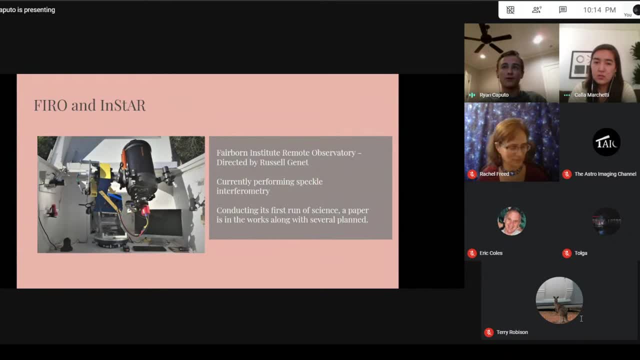 And FIRO, which is the Fairborn Institute Remote Observatory directed by Russ Jenae. He has a more permanent installation, which you can see here, That is going to be doing lots of speckle interferometry, Something that's more than just two or three nights. 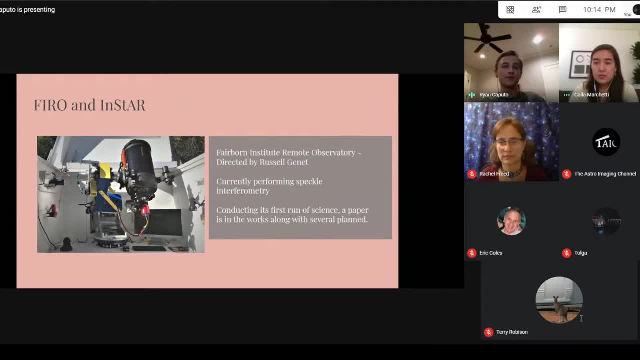 Two or three nights of observing runs. This is going to be doing observing runs, hopefully every night, And hopefully somewhat automated, so I don't have to stay up every night, Although I could do that regardless. It's currently conducting its first run of science. 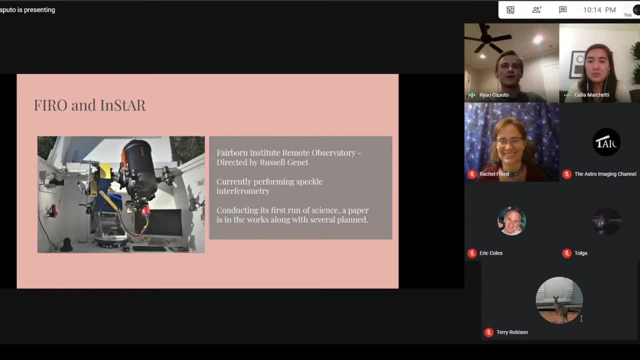 We are staying up quite a bit doing lots of double stars, And we have a preliminary paper going, And Russ has several papers down planned, And so we have quite our work cut out for us, Which is great. But seriously, though, we actually really enjoy doing this. 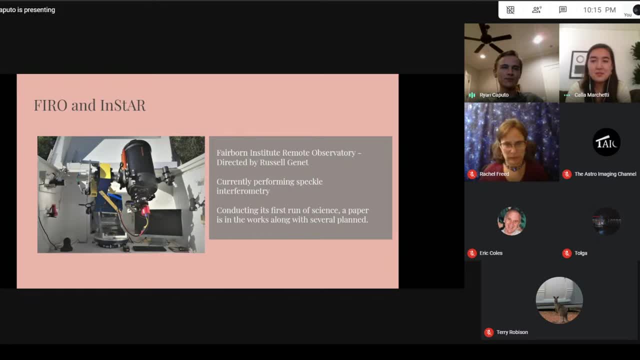 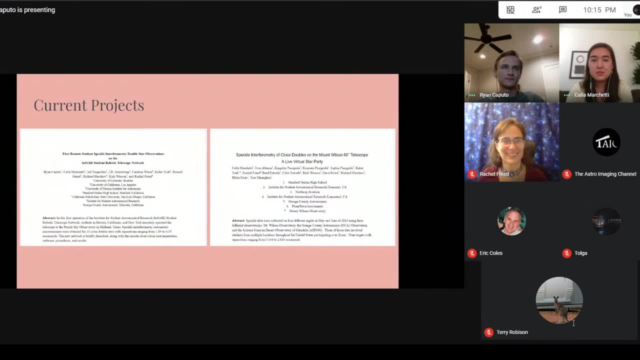 It really is fun Because this double star research- it's amazing to finally break through the seeing limit And be able to measure double stars. And here are some projects that we're currently working on. There's the first remote student speckle paper. 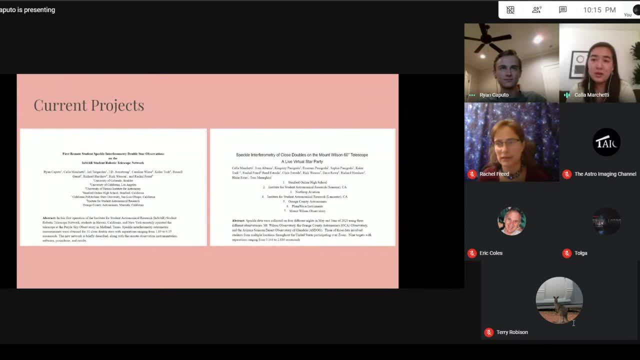 Which the data is from the observing run that Ryan, Caroline, Jed and I got. And so that's about it, Those 31 stars, And we talk about remote observing And the software used And we do some data analysis where we compare our measurements to the historical measurements. 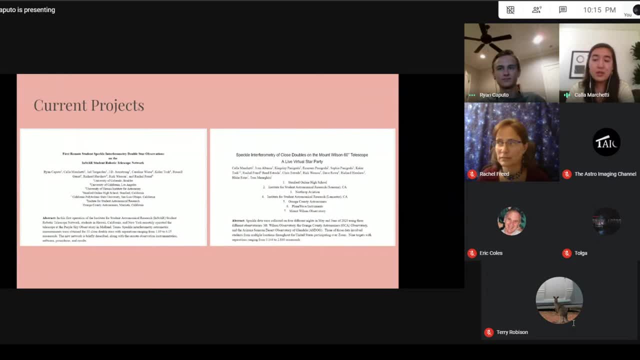 And we also look at how our data compares to the LCO 0.4 meter telescope And we, even though the LCO telescope is a lot bigger, speckle interferometry more than makes up for that And it results in clearer images that we get. 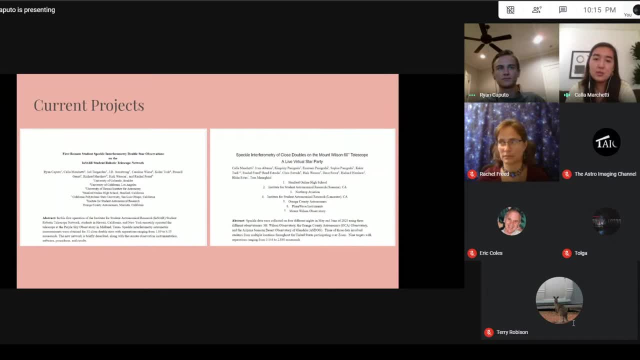 For close double stars. And then there's also the another paper, and the data is from the mount Wilson 16 inch telescope, As well as some data from other observatories in the instar network, And with the 16 inch telescope you can get to stars with separations of 0.1 arc seconds. 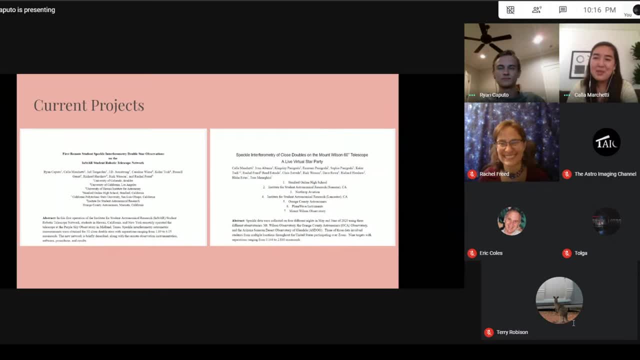 Which is a lot closer than the 1.89 that we were so excited about, And when you have stars this close, Their orbits are much shorter. So we were able to look at stars where orbits have already been observed and completed And we were able to compare our measurement to the ephemeris and see where the position should be. 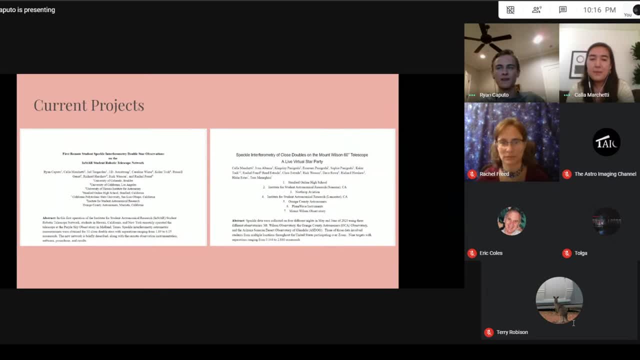 Compared to what we got. Yes, And looking forward. there's a lot of opportunities with the new Gaia data release. Well, it's not necessarily new, But there's so much data It might as well just be new As well. 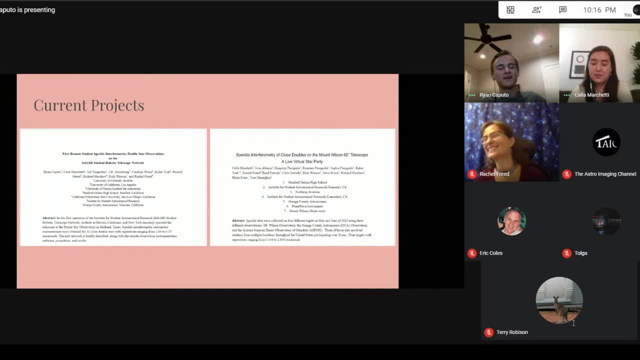 Because we barely scratched the surface of it, Dave Again showing up. He has written a program, the Gaia database search tool, I believe GDS, Which he compiled. all the double stars that can be identified in the Gaia catalog. 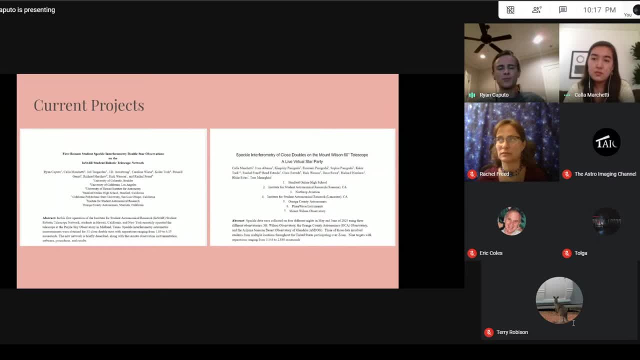 So with ones with similar parallax and proper motion. And a lot of these stars which look like they might be orbiting are not in the Washington double star catalog And many of these are in the 1 to 5 arc second range. 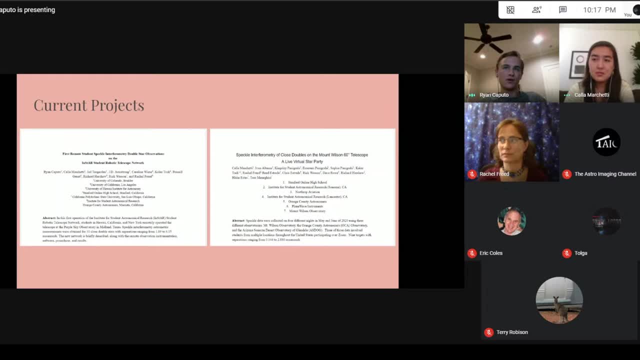 Which is the perfect range for speckle interferometry, And there exists a need for measuring all these double stars And INSTAR is working to develop a program to measure these stars at large and do a very large volume study of that. And then I first got into research with astrophotography. 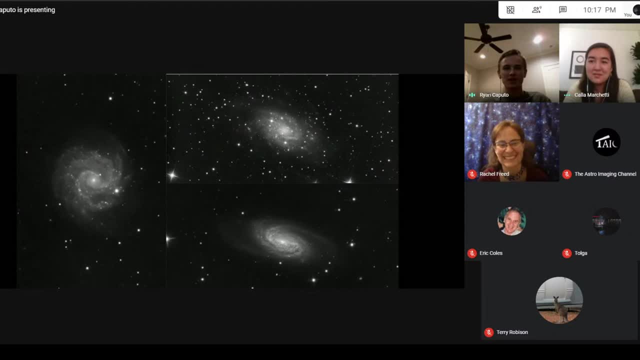 So I figured it would be suitable to show some of the pictures I've taken. I remember a long time ago I took a picture of a star cluster, But my mount didn't go too properly And so all it was was just a random star field. 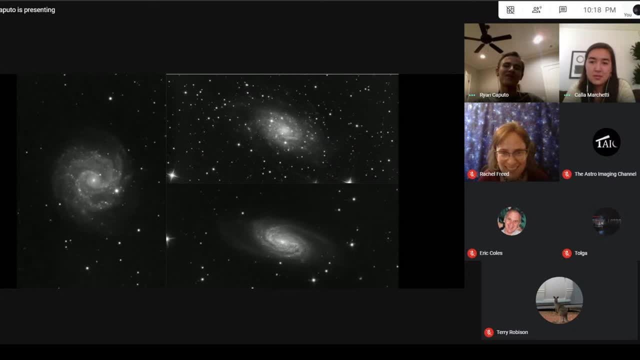 So I was pretty bummed And then I saw a double star in the frame And I asked myself a question. I said: can I measure this double star and can I publish a paper? A single question. A single question was the wrong question to ask. 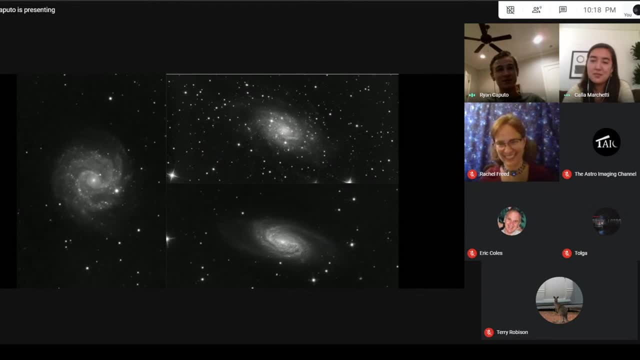 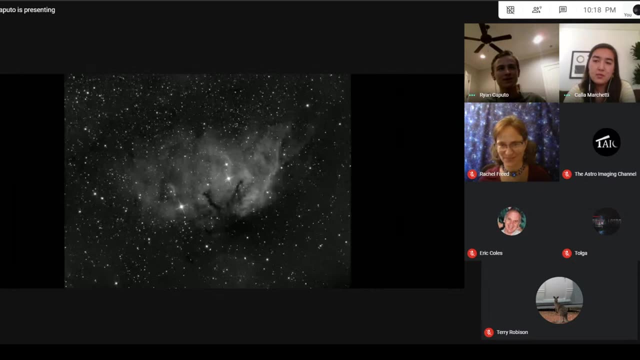 That let me down quite the rabbit hole, As well as the rabbit hole in astrophotography, And this was all taken with my 6 inch classical caster grain And this picture I'm particularly proud of- It's the Tulip Nebula. 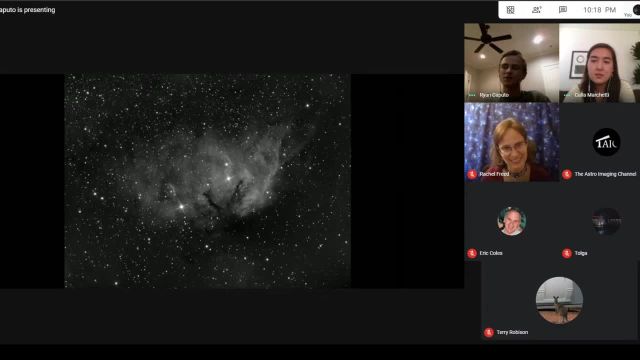 I actually took it over July 4th, So pretty recently. And just thinking back, Rachel Russ, my teacher, Kalei Talk, Who's also affiliated with INSTAR, She's the vice president Alongside Rachel. They really give me a lot of options and a lot of opportunities. 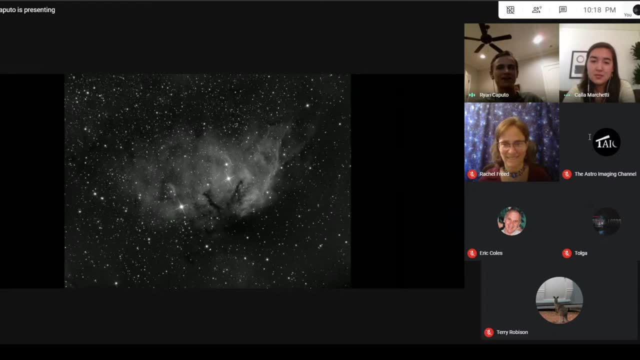 And it's been amazing to work with these people And to It's so satisfying To have each of your projects and each of your papers To see a progression, to where you look back and you say, okay, This paper, I started out in this paper. 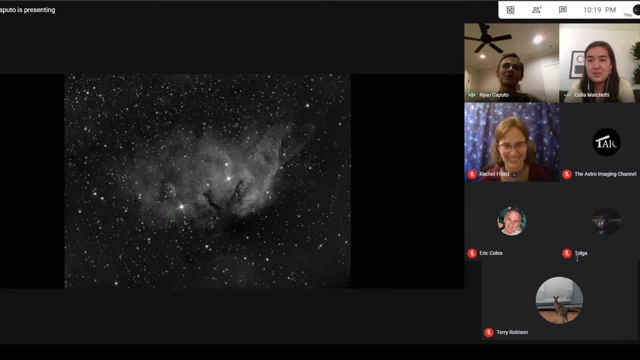 I did more and you know just that satisfaction, Knowing that you're doing more each time And progressing in a field that was originally an intro, Because Rachel mentioned double stars are like the: The easy, the easiest paper to do. You know, being able to take something like that. 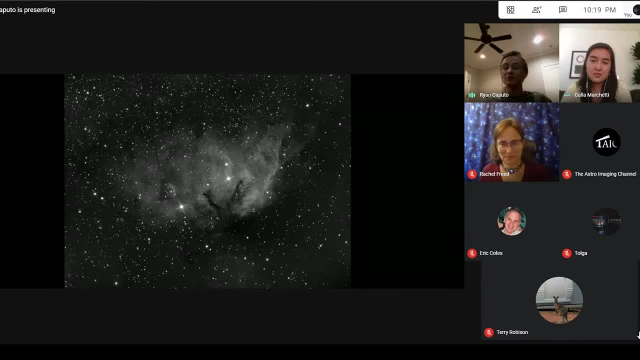 And go to a point That is much further is very satisfying And very grateful that Rachel has allowed that. So A couple more questions. Okay, I think the question has been answered, but the objective is to get The exact separation between the stars. 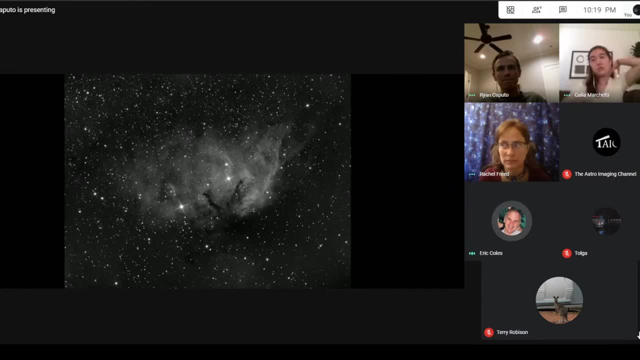 But, Rachel, I answered that it's for astronomy, Strong Astronomy. I'm sorry, I almost didn't get that out, Rachel, Sorry. Yeah, Could you just clarify that. Give us a couple of minutes on the objective And, by the way, you guys hand off the presentation better. 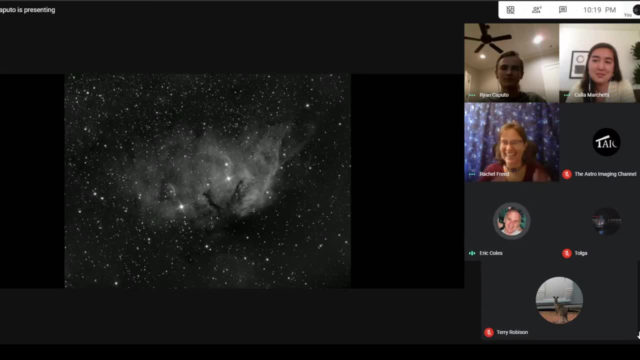 Anyone else I've ever seen. You have a clue? What's the signal? What's the signal to hand off between your two presentations? We'd want to know. I digress, You can answer the first question. I appreciate it. Yeah, well, we just got it down, Cal and I. we just went through it. 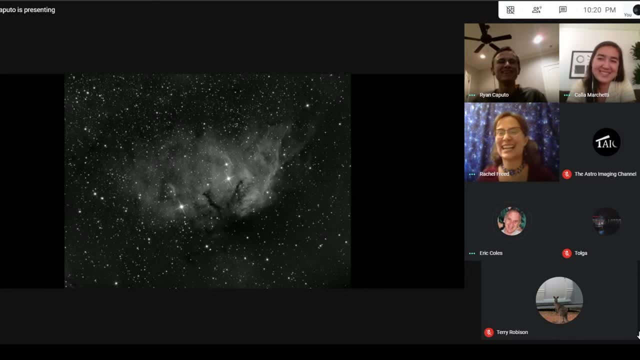 So, Like I mean, there's a lot of different things. I'm sure you've all been in the same room 30 minutes And you know memorize. Okay, I'll talk here And you talk there. 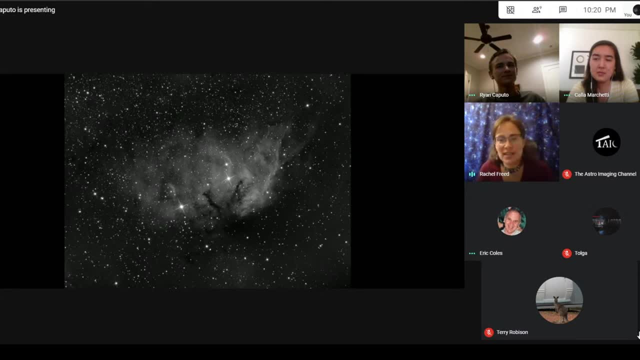 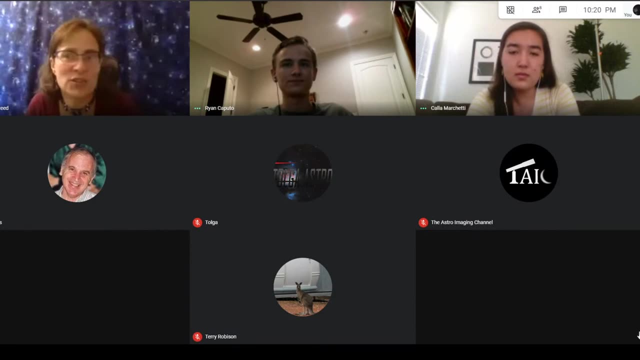 Rachel, do you wanna answer that question? So the, the Astrometry, we are just measuring The separation and the position angle Between the two stars To add to what What's already known: So many of the stars that we have studied. 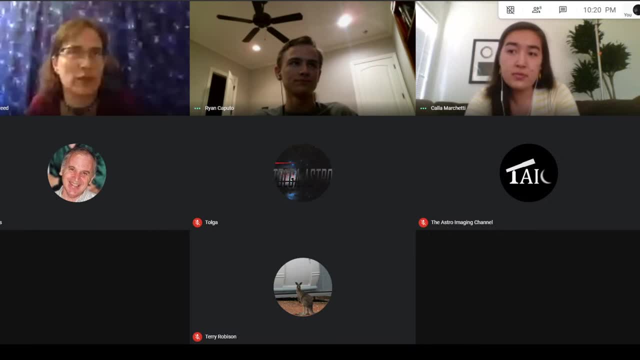 The past. You know we're first discovered and reported by John Herschel and and others. you know hundreds of years ago, 200 years ago, but we're sort of adding to the databases of positioning stars, hopefully finding ones that are orbiting, and and use that information. 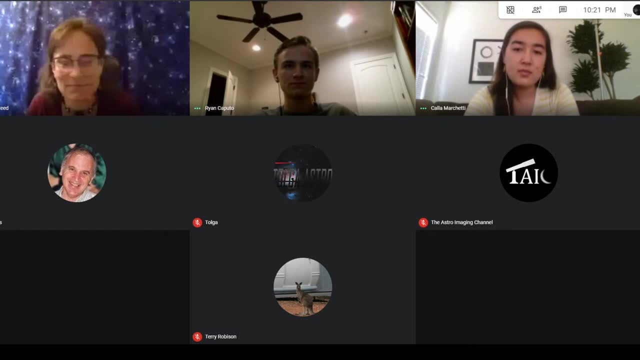 of course, can then lead to masses and everything about stars. But yeah, the goal is to measure the position angle and the separation of the two stars. Do you ever just scan your photographs or just go hunting for new double stars and haven't been discovered? 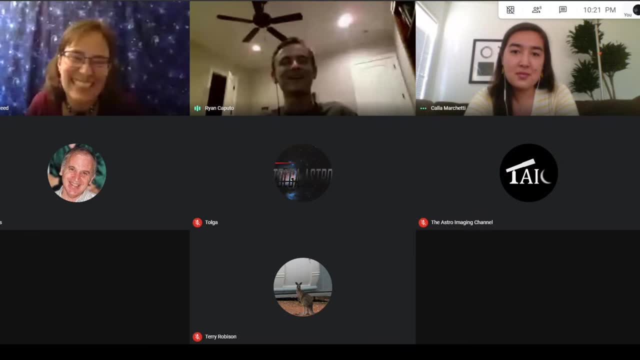 Brian, I can say something about that. yes, Oftentimes I will. in my astrophotography I will go through the pictures and and note stars that are close and I'll go to the Gaia catalog and see if they have similar parallax and proper motions, and oftentimes they do, as in they 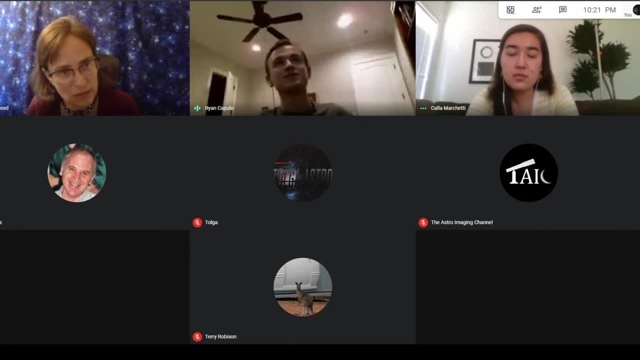 could possibly be gravitationally bound. And there's this one double star that I think is found. It was like magnitude 17, is some really faint star in the corner of my image in this galaxy clusters is in the foreground and it looked like it was gravitationally bound, but it did not have a WDS number. so, yes, there are double stars all over the sky, everywhere. 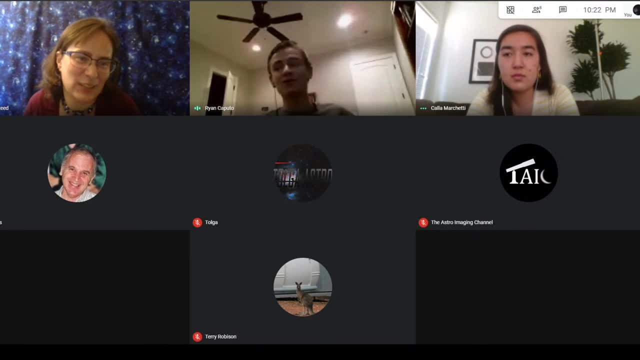 that are not measured- not in the WDS- and I encourage all of you to look through your images and check for these double stars, and if you find a double star, Maybe write a paper of it and you can discover a code on it. 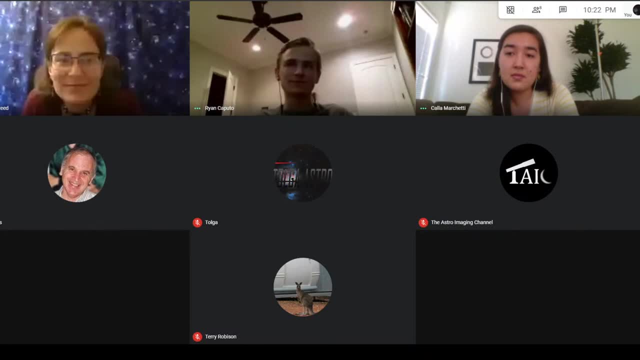 And didn't we? didn't we kind of learn that over half the stars are really double stars? Yeah, Yeah, A lot of stars are doubles. however, not many are doubles that we can measure, because if we're looking at a four arc, second double, because astrophotography is going to be seeing limited four arc second. five arc second is about the limit there. Anything over that separation is automatically a very wide star. You know A thousand astronomical units, So a lot of stars are like spectroscopic binaries where they're so close. you can't even resolve it with Hubble, It's just, you only see it with the Doppler shift. 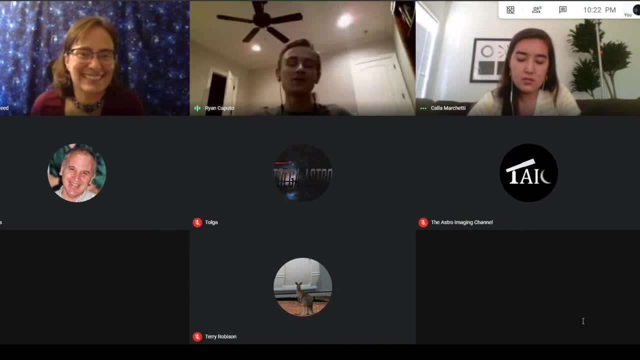 So, although a lot of stars are binaries, not many stars are binary. so we can measure. And how do you differentiate between a true double star and one that's where it's just parallax, Like an optical, like where you see two stars in the sky but they're not actually orbiting? 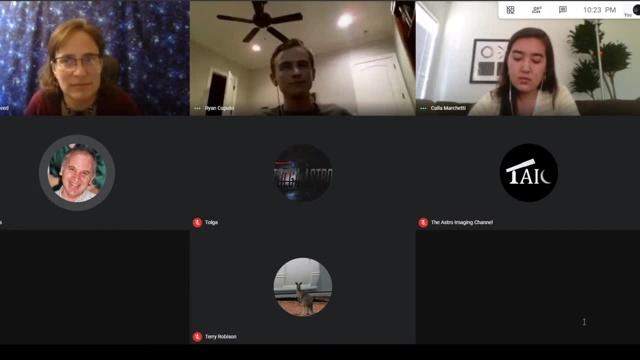 Right, they just happen to over, mostly overlap, and they might work to be a double star to you, right? Yeah, there's actually no way to tell without using the amazing catalog provided by Gaia, because they look like two stars, Really look like a double star. If you go to the Gaia catalog, you can look at the parallax motion or the parallax values, and that tells the distance, the stars and if the parallax is at the same. 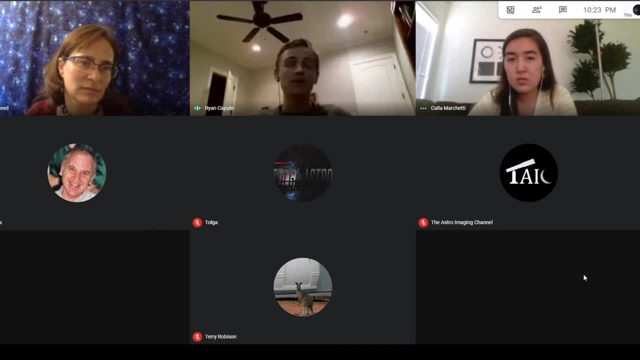 The distances are the same, and then you can also look at proper motions. If the proper motions are the same, they're moving through space at about the same velocity, which means they have the potential to be orbiting. The only way to actually confirm a double star is to take measurements of it and then maybe 100 years later, after 100 more measurements, then you might see an arc, and that indicates that there's some gravitational relationship. 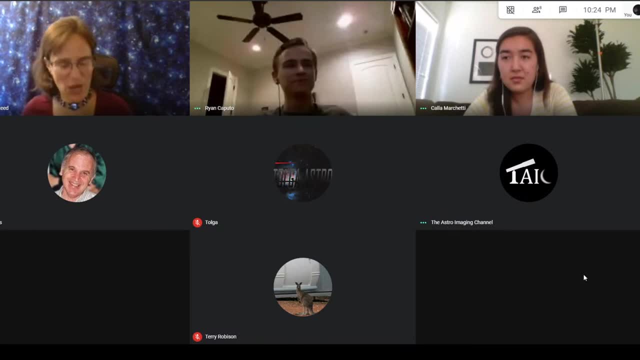 But otherwise there is no way to tell if a star is a double Or a double star. Sorry, if the star is true binary. I have a couple of questions. One is: everything that you were using, including the software, is available to amateurs. 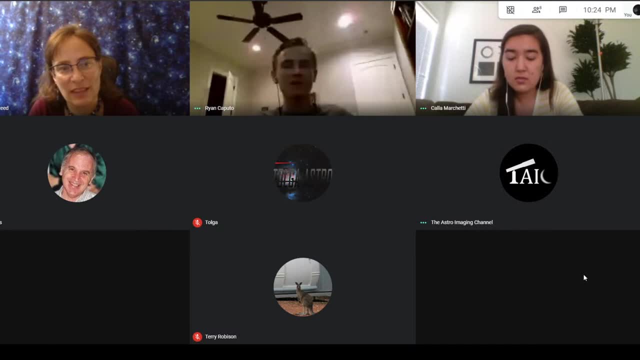 This is, there's nothing. there's nothing fancy there. Yes, Okay, Um, the software you were using, the speckle software from plane wave That's. is that a free download? also, That is free. However, it's not down. you can't download off the internet. you're going to have to email Dave row for a copy of the software and you will provide it. 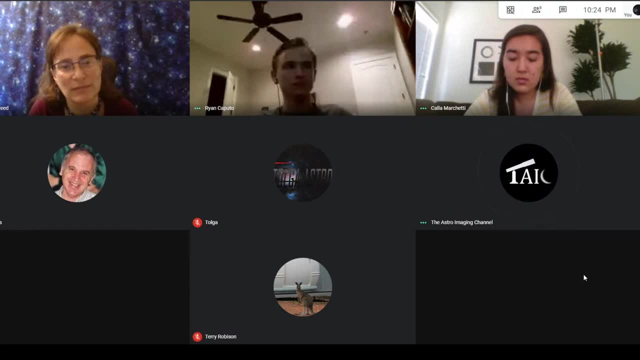 Okay. Have you ever played with a with a three star system? What happens then? I There. actually, that picture that I showed in the slide was a three star system, I believe At the beginning. It gives very strange results with auto correlation. You get like duplicate, because those sidebands get duplicated for the tertiary like I think, twice. so you have like six stars. I'm not actually totally sure. Kelly might know more than I with this, because you mess with that data a lot more than I did. 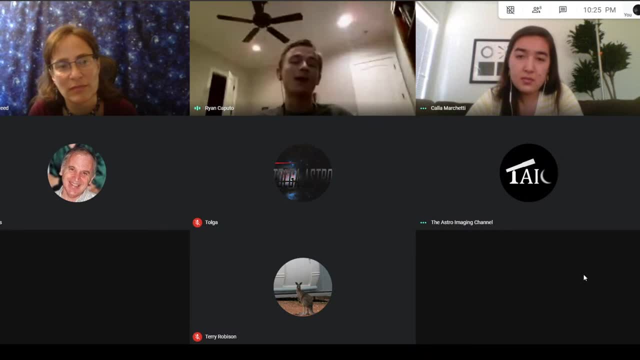 But yeah, triple stars get kind of confusing, and for that that by spectrum processing, which I briefly mentioned, is better suited, because that gets you the actual input, Because that gets you the actual image, And so it's a lot easier to not get confused: which is which. 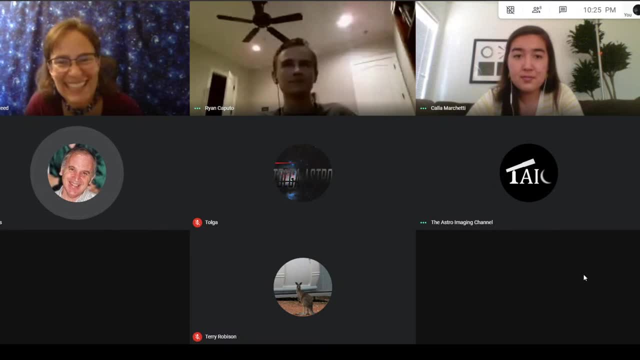 Thank you. I have one more question. This is interesting, so my mind is is working, which is pretty rare this time of night, but do you ever go to some of the space telescope data and look at that information? they obviously don't have atmosphere issues. 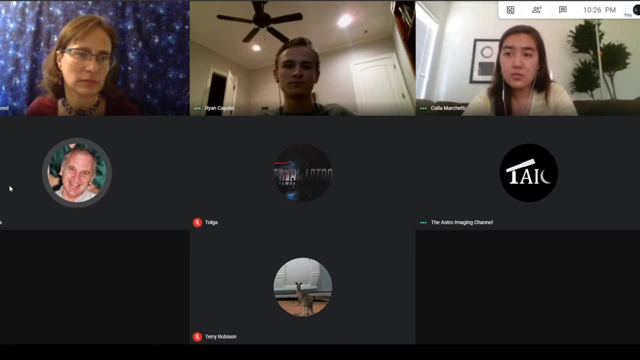 They can probably resolve double stars- I don't want to say easily, but certainly better than ground base. Yes, the parkos satellite that did a lot of resolving and I'm not sure who did it, But there was this publication of some sorts that published all the parkers data into double stars, and so if you look at historical measurements for double stars, 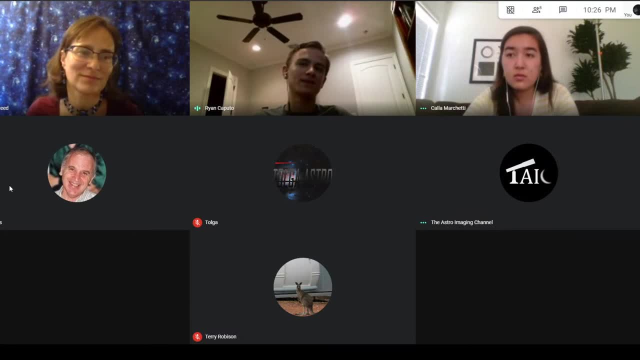 Oftentimes they will have an H For parkos and that's that telescope making that measurement and there's only one measurement, because it only measures for once. Gaia does not have that, although I believe, Rachel, you might have some knowledge about this. there might be an initiative to get some guy data into the WDS. 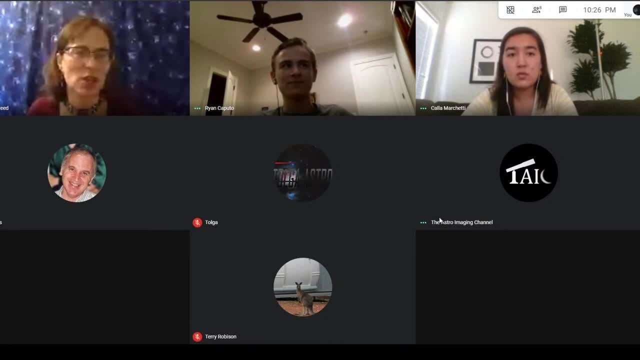 You know that's going to happen. Yeah, I think that's sort of a slow process that has to be published first to get into the WDS. I'm not sure. I'm not sure how that's working. Well, um, yeah, that there might be some time in the future we might pull up a plot of the historical measurements and they'll be a G for Gaia or something. 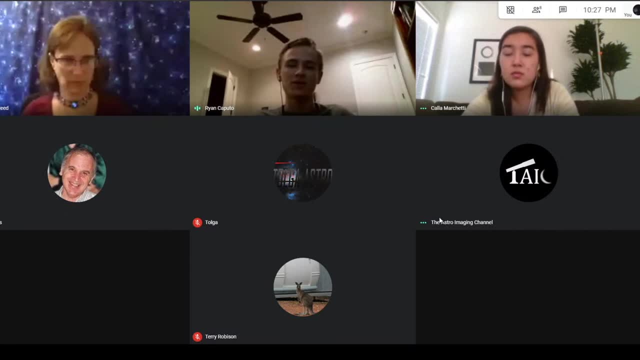 Yeah, I don't know. But yes, you can go and look at data straight from the in the catalogs and you can find double stars using that, which is what Dave Roe did with his Gaia search tool. He he didn't start with the WDS, he started with the Gaia data and then said, okay, this star from Gaia is this WDS star. 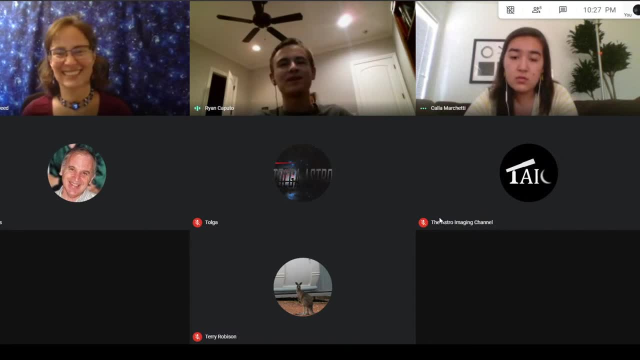 from Gaia doesn't have a WDS number, So it has been done before. yes, So to your question earlier, if students sort of goes through just through their images and looks for stars, I'll say there's a paper that's probably going to come out in the journal double star observations in the next issue or two, where students actually 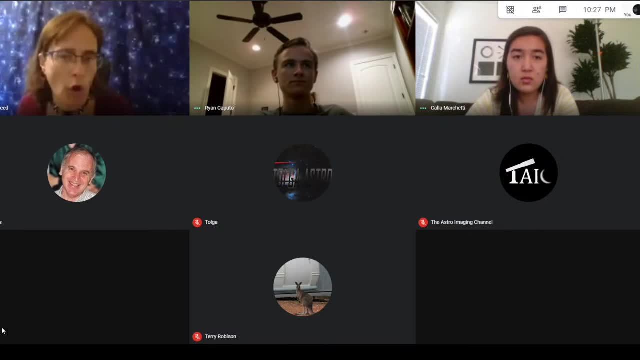 selected a double star to study. They took images but couldn't resolve the two in the images they got but noticed two other sets That looked like they might be double stars and they ended up, doing their research on those two pairs of double stars, figured out that one of them could potentially be a binary system based on Gaia data. 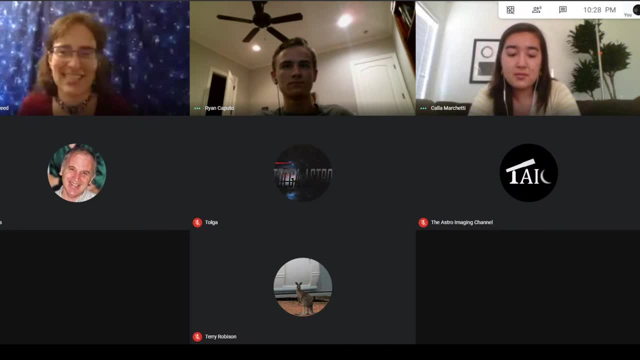 So other students definitely have been doing that as well, which is really exciting. Alex, I think I'm all set here. Okay, Do you have more things that you would like to tell us about tonight? And anybody out there That's got on YouTube? 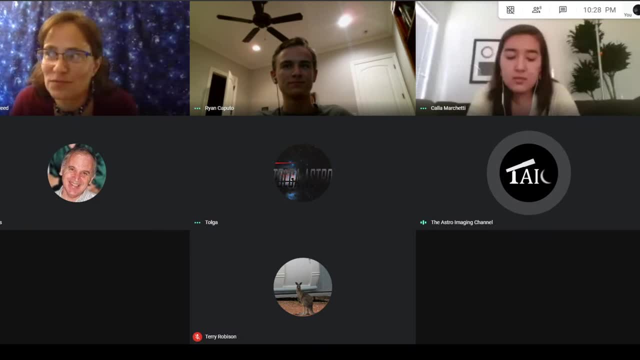 Be sure to get your questions in, because we're going to start wrapping up here. Rachel and Ryan and Carla, do you have something else you'd like to tell us? Um, I just wanted to kind of mention- to wrap it up and bring it to a close- that this is kind of amazing work that started from just as simple- as Ryan kind of talked about, a simple double star project- to now something that's all encompassing of their lives. 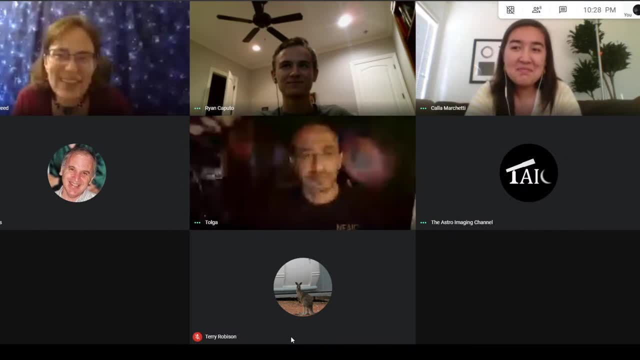 but is really being transformative, And they're helping to build a robotic- as student, robotic telescope network for research that will be 100% dedicated to you know this, this process and what the students are learning. it's not just about making this measurement measurements. it's about learning how to write and communicate scientifically, and I think we saw that they know how to communicate scientific information pretty darn well. 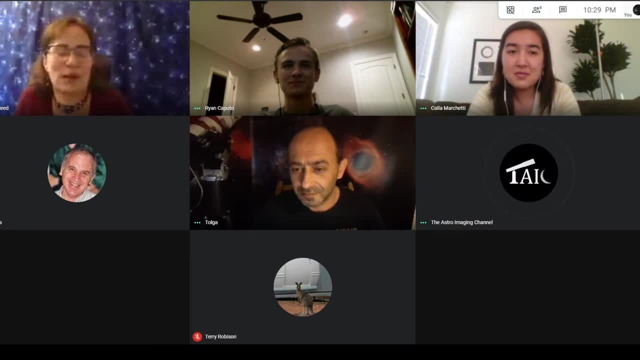 But the fact that you know they're having, they're going to have, several published papers. Ryan already has a couple. I don't know about everyone out there listening and watching, but if you think that first time you published a paper, if you have published one- I know I wasn't in high school- 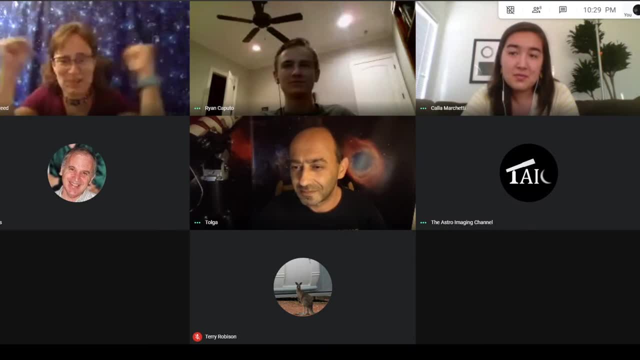 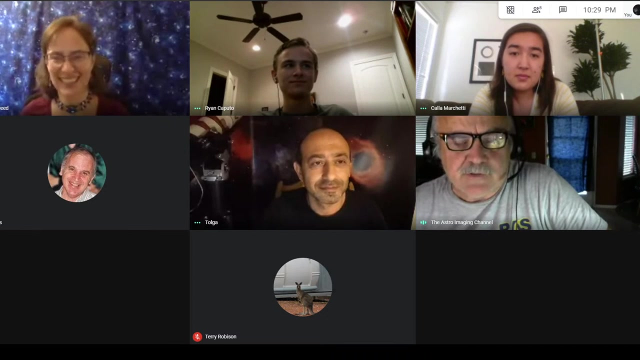 When I first published and it's just an amazing process and rock. Thank you, And thanks for inviting us to talk. you guys, Thanks for coming And I'd have to say that if one of the goals of this program is to enable students and others to learn how to communicate, 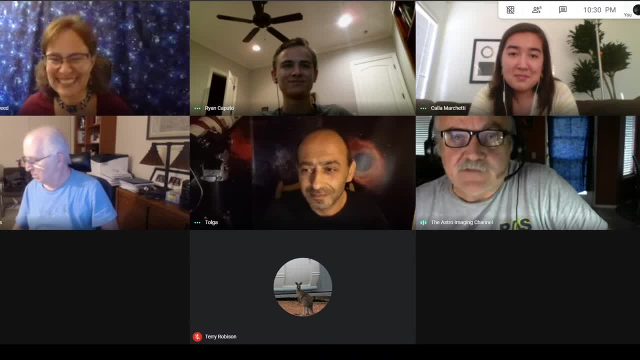 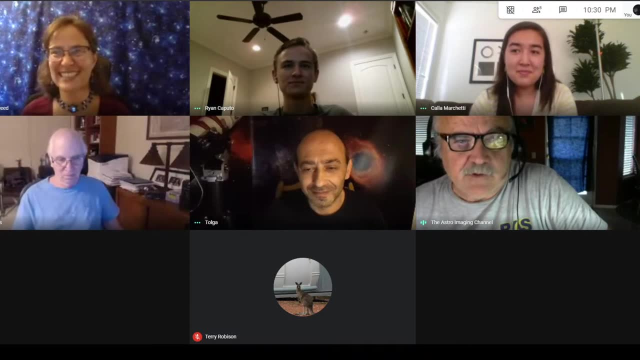 Well, you got a couple of winners there, That's for sure those. they're very smooth presentation. You guys did a great job and it's got a couple of good comments. I'm going to share my screen a little bit now, If I can figure out how to do it again. 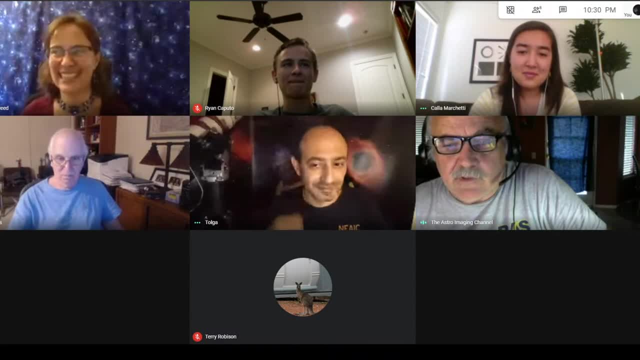 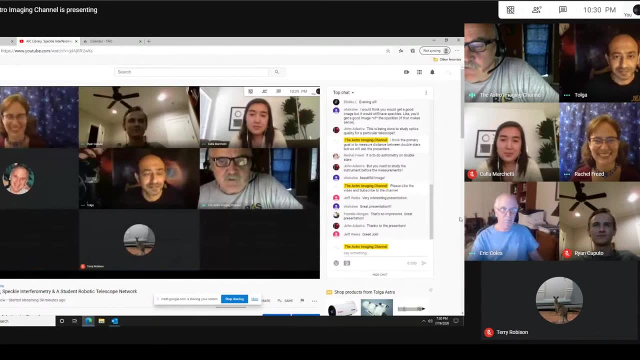 Share my entire screen doing share and head over here. As you know, there's a big comment section over here where you can ask any questions and if you've got any questions, get them in quick because they're there, Okay, Okay.